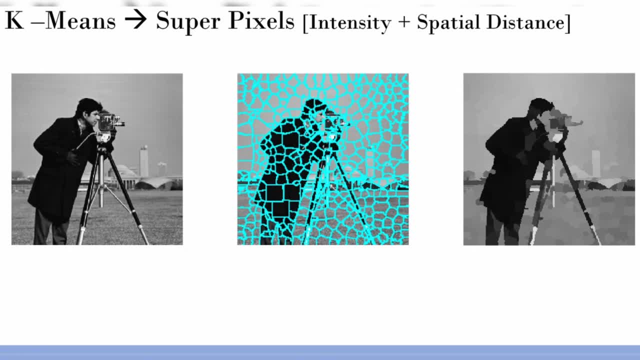 Or maybe you start with the highest intensity point in the image And then you consider the neighborhoods, expand it based on a threshold. You come up with a segmentation till that expansion converges right, So that's region growing. Then we discussed also about region splitting and merging, where actually you start with the entire image. 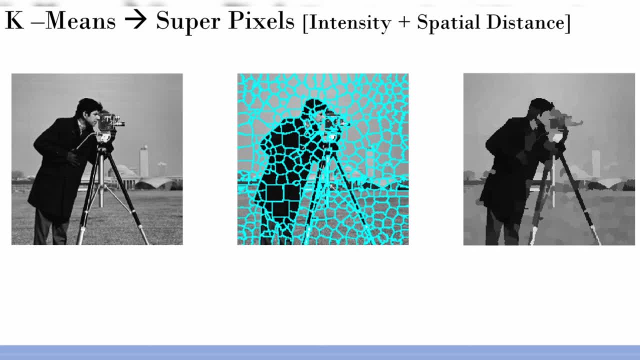 You split into small segments, small quadrants, And then you see individual quadrants And based on a threshold or maybe something like mean or variance, we will group them together, We will merge them together And that's why It's called split and merge. 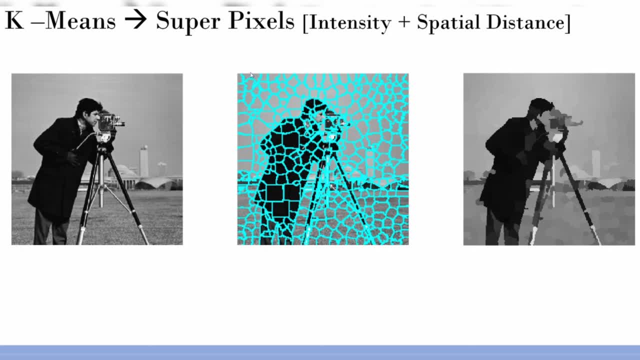 And then last we discussed about this beautiful technique of super pixels. So here it's actually k-means, but k-means extended to the distance also, Because earlier it was only intensity. Now you will consider, let's say, I start with this cluster. 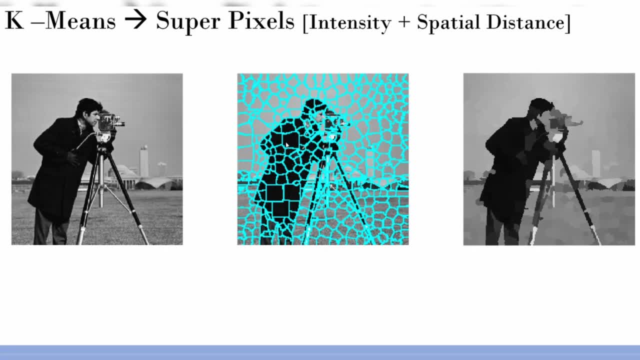 I will consider a region around that, So I put a threshold, So nothing beyond that. So two conditions have to be satisfied. to be frank, Just to reiterate what we were discussing, Two points have to be considered. So one was actually the distance constraint. 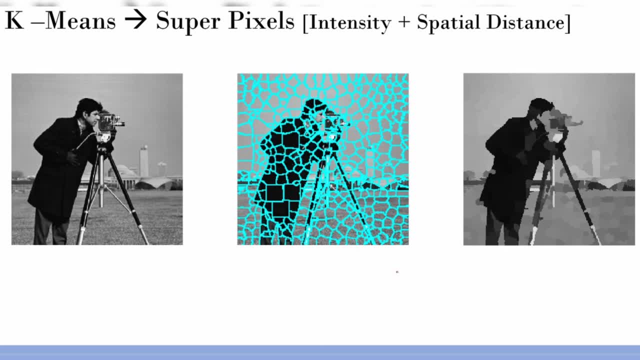 So sorry, the intensity, Intensity constraint, which you could actually put it in this way. let's say d, so basically two distances, right, You put. let's say you can put color or distance, So let me call it. I mean intensity. 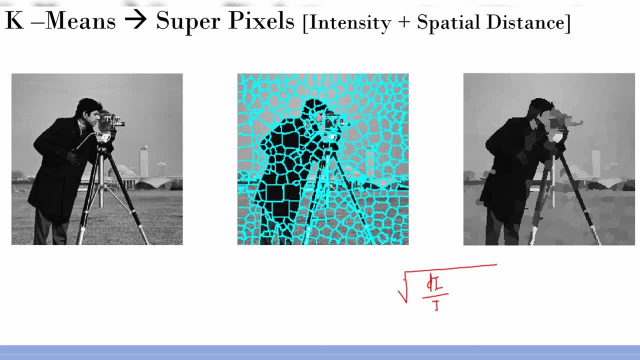 Let me call it as di by some intensity normalization, Or this can be actually dc by c, ok, So whatever it is. So this is on the intensity side, And then you put another threshold on the distance right spatial side also. 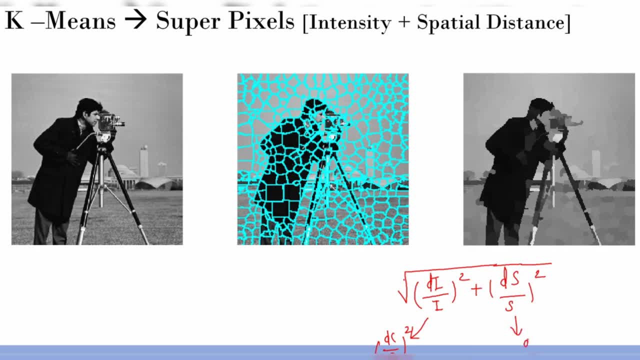 So this was the expression we were minimizing. So this is basically on the distance spatial distribution And this is on the intensity right And just to expand. I mean, if you are confused, basically di is nothing, but let's say your. 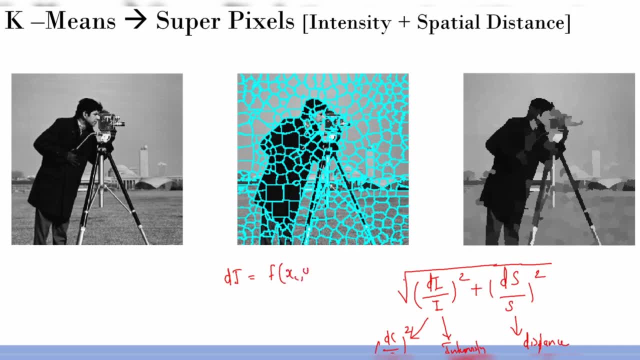 centroid pixel is something like: let me call xc, yc, This is the centroid pixel. Then you will consider that to all the other pixels- xi ya, neighborhood pixels, basically right. And then what you do is basically see the norms right. 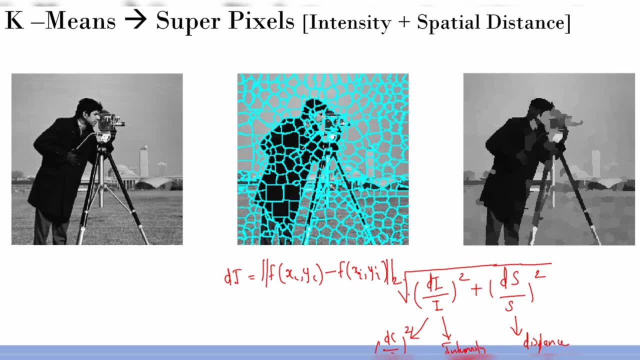 Mean square, sort of error, sort of thing. right, So this is basically di. And then of course, this ds is nothing but again same, if you consider. it is the spatial distance, So xc minus xi square, the Euclidean distance plus yc minus yi square. 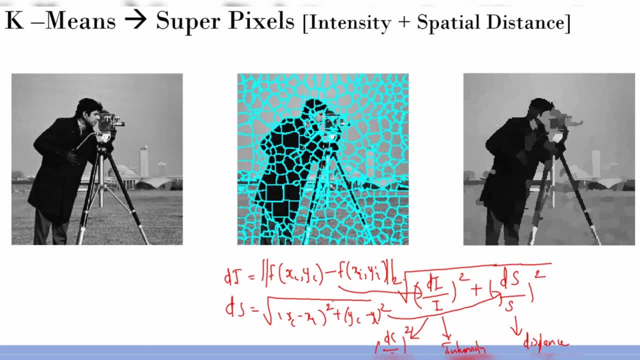 So this is your ds right And this is your di. So only problem here is di And di is basically in terms of intensity. ds is in terms of intensity, Ok, In terms of distance, maybe millimeter, for example. 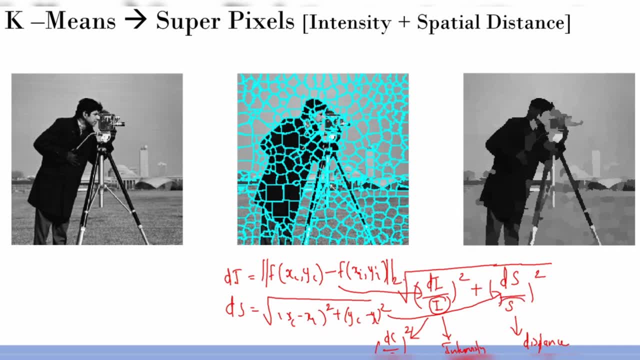 So they are two different entities, So you need to have this normalization factor so that they can be added and together can be considered as a sort of a constraint, right? So this is the idea in super pixel And that's what the result you're seeing over here, right? 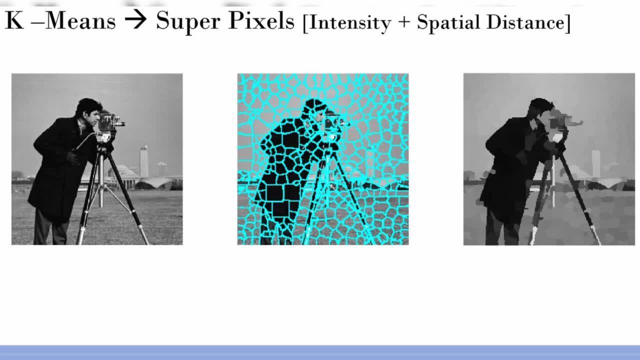 So the basic motivation towards super pixel is something like: instead of starting from millions of pixels- original pixels in the image- you start from some super pixels, which is like a subgroup of pixels Right For any further. So this can be standalone as a segmentation. 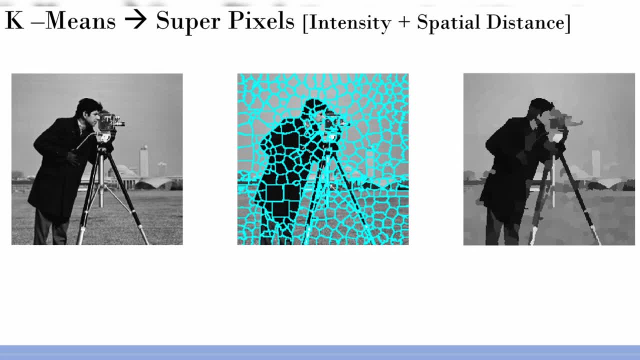 This can definitely work out, or it can be used as a seeding point to another segmentation. Ok, So even some of the techniques, like the next one we are going to discuss, actually uses super pixels as an intermediate processing. Ok, So let's move on. 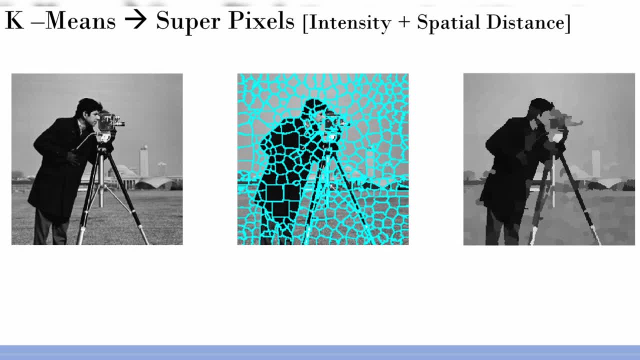 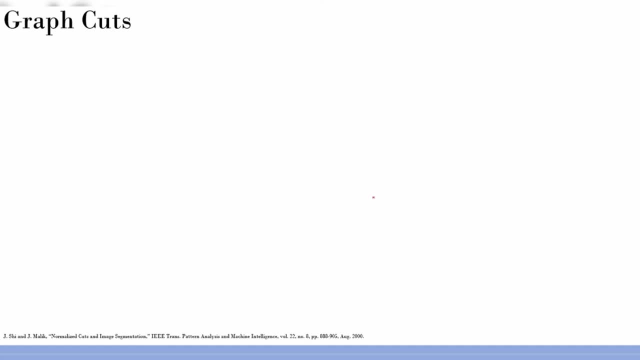 So now we are going to the last section on in this week, which is the most interesting one, And I love this topic And, in fact, those who are coming from graph theory will appreciate it much more. Even I am not really from graph theory, but still it is a very interesting approach And this was proposed. 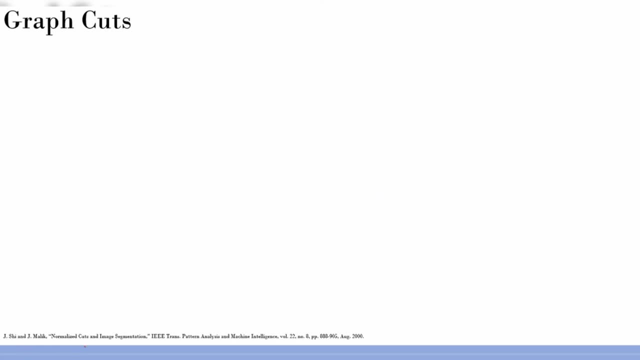 by Shi and Malik in 2000 in IEEE PAMI famous journal, And the idea here is actually you convert the image segmentation problem into a graph, theoretical problem or graph. You convert image to a graph and then you basically try to cut the graph using some criteria and 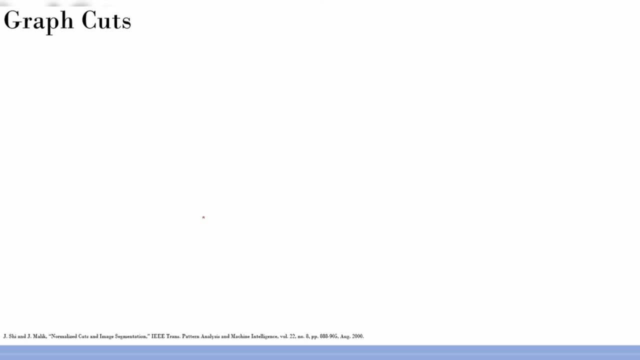 by doing that you have a foreground and a background. People have extended it to beyond two class segmentation, beyond foreground background segmentation, multiple objects or semantic segmentation, for example. But let us actually concentrate on a two class problem where I want to segment the image into a foreground and a background. So the 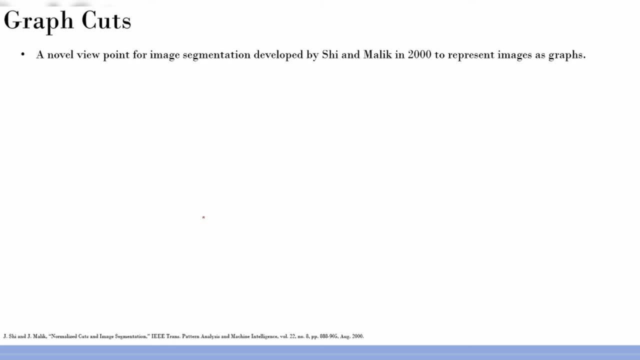 idea here actually, as I said, it is a novel that time when they proposed this. So the idea here actually, as I said, it is a novel that time when they proposed this. So the idea here actually, as I said, it is a novel that time when they proposed this. So the 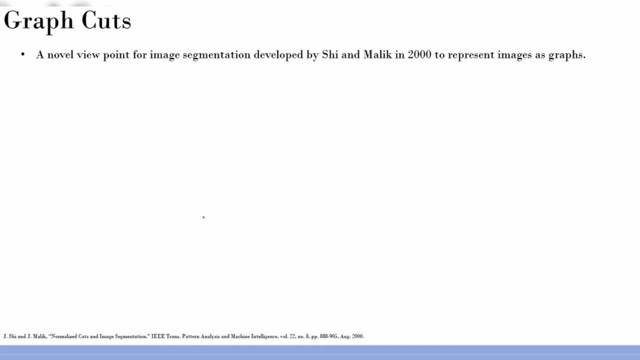 way that they proposed in 2000,. it was a novel thought process. You extend image segmentation into a graph, theoretical problem. So that is the interesting part. And in fact, if you see image boxing, segmentation particularly different approaches have come across Something. 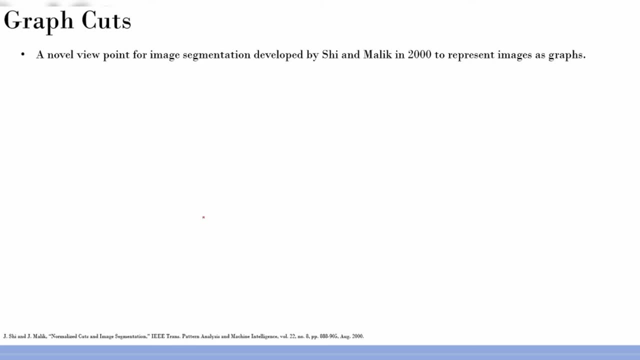 from graph theory, something from partial differential equations, which you will see later next week, And so many other ideas have come from different areas. Okay, so that is the beauty about image segmentation, because the way you are going to approach segmentation problem can be different perspective, and one such perspective is the graph. 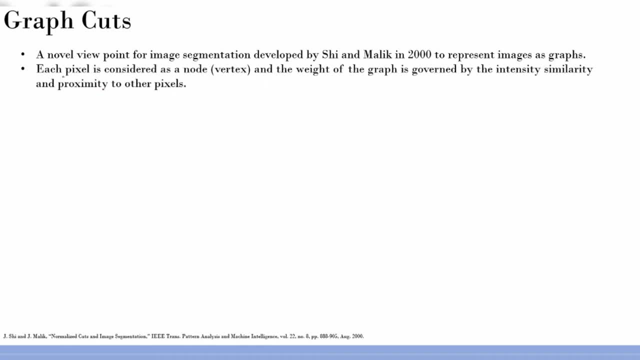 cuts. ok, So what essentially we do is each pixel in the image is considered as a node in the or vertex in the graph. ok, So you have graphs right. So the graph will have a vertex or a node and an edge right connecting to the other node or vertex, right? I mean, basically this is the concept. if 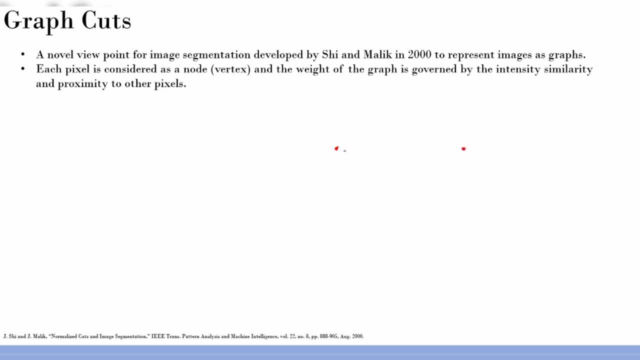 you are confused. So this is a node or a vertex, and this is another node or a vertex, So this has to be connected two aspects. So these are nodes, right? or these two are the nodes, and then this is the edge, and edge will have a direction also and a weight also, right? So that's. 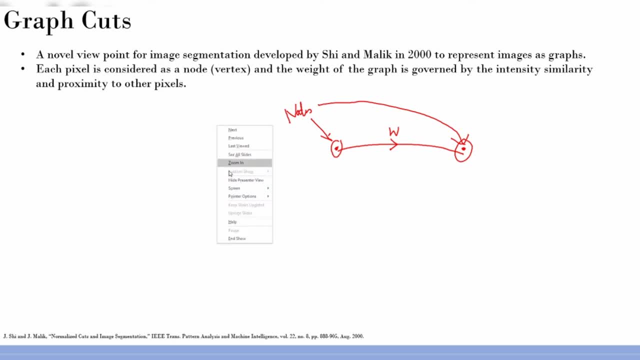 what essentially we mean. So a graph is basically consisting of a node or a vertex and an edge which is directed. ok, And in our case, in the case of image processing, image segmentation, each pixel is a node or a vertex and the weight, the connectivity between the pixels will be. 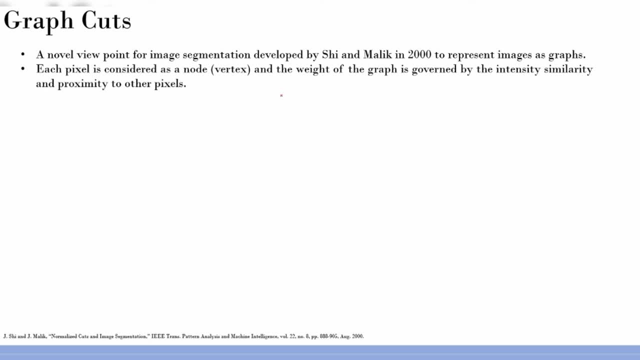 having a weight. and of course, you can put a direction also The direction. I will explain what is the direction here, what we mean by direction. and of course, the weight is governed by the intensity similarity. ok, So you, if you are closer and your intensity is similar, you will have 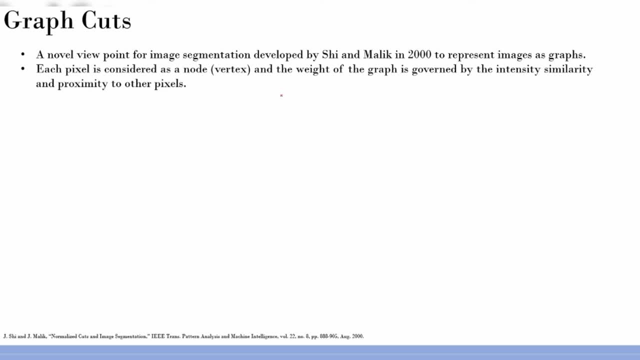 higher weight? because they are. they seems to be connected. ok, So I will explain this. don't worry, all I will put in the equations and it will be very easy for you to understand. ok, So the concept is simple. you consider the images, then you consider each pixel as a node or a vertex, then 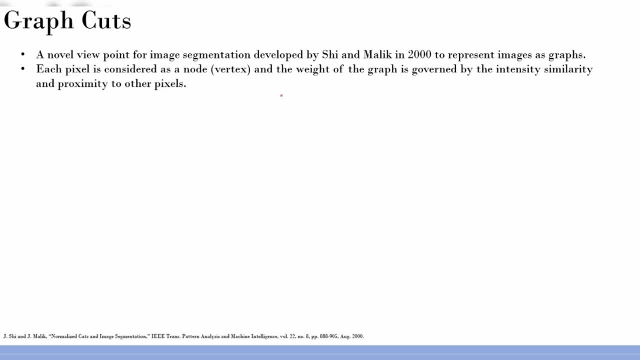 the connectivity between the pixels is the same. So this is the concept. So the concept is simple. you consider the images, then you consider each pixel as a node or a vertex. then the connectivity between the pixels can be measured in terms of its similarity and the distance from the other. 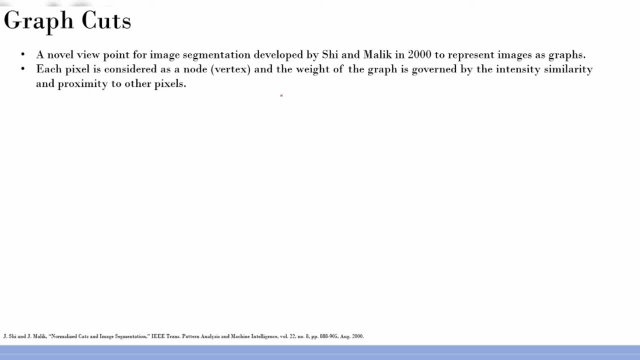 pixel and that is the weight, ok, and there is a direction also associated with that. And the interesting part about this paper, which came in 2000. you see the number of citations, ok, So this is one of the highest cited papers in image segmentation and I encourage all of you to. 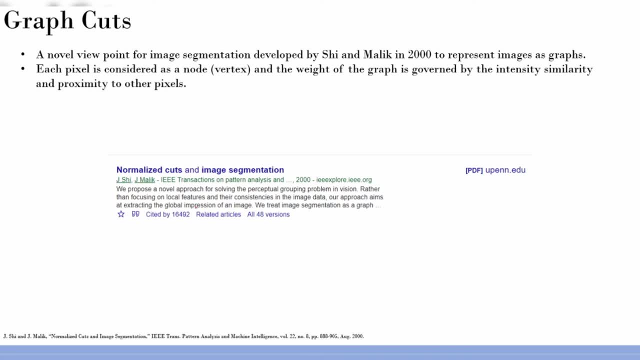 have a look at it. Slightly difficult if you are not coming from the graph theory to really go through it in one shot, but you will understand it. the concepts are very nicely explained. If somebody is really interested in this then you can do it. So this is the concept. So this is the concept. 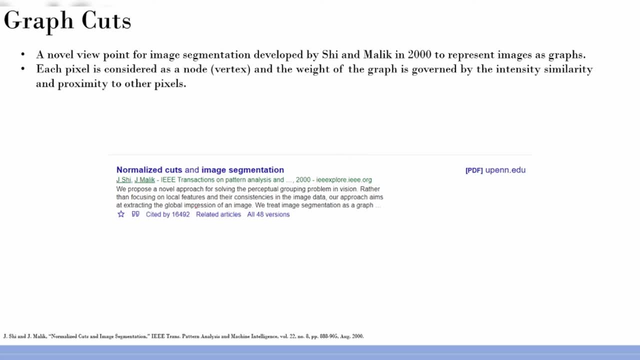 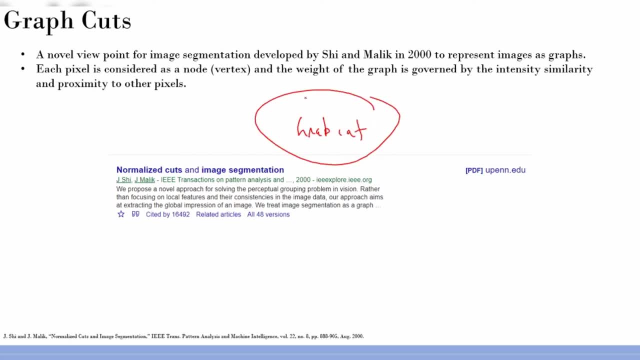 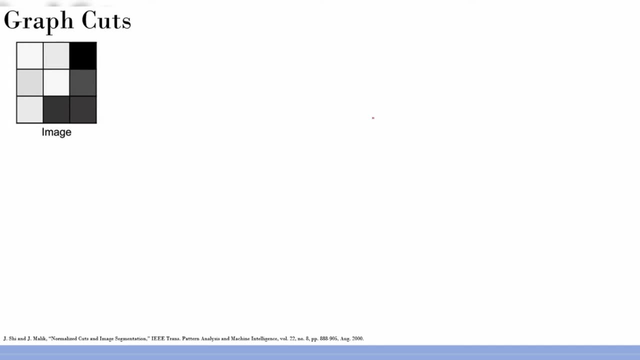 right graph cut. This is actually inspired from graph cuts. ok, So let us move on. So let us dig deep and see what is this beautiful technique all about? ok, So this is an image. let us assume again an illustrative case. So you have some white shade here and you have black shade here. Ideally, you want to separate this part of the image. So you have some white shade here and you have black shade here. Ideally, you want to separate this part of the image. So you have some white shade here and you have black shade here. Ideally, you want to separate this part of the image. So you have 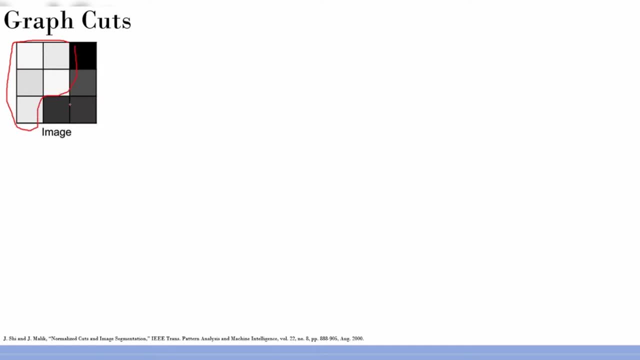 some white shade here and you have black shade here. Ideally, you want to separate this part into one segment may be foreground and the other one into background, right? So that's an aim for us. Of course, it looks so easy as a human, but if you have to automate it, that's a tough part in many. 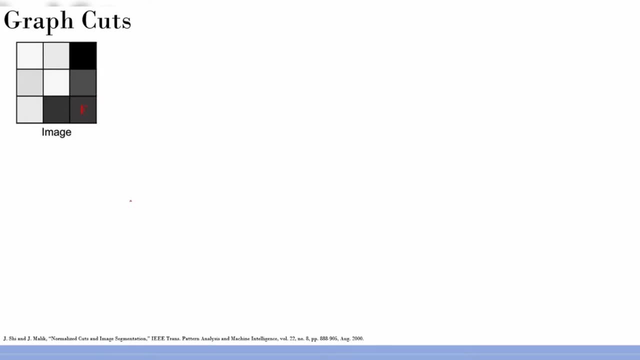 cases. So what we do is we convert this into a graph. ok, and let's assume: ok, for the sake of simplicity, let's assume this is foreground. ok, So the black shade is the foreground and I will mark these pixels as a foreground. let's say, ok, So this is foreground and maybe this is background. 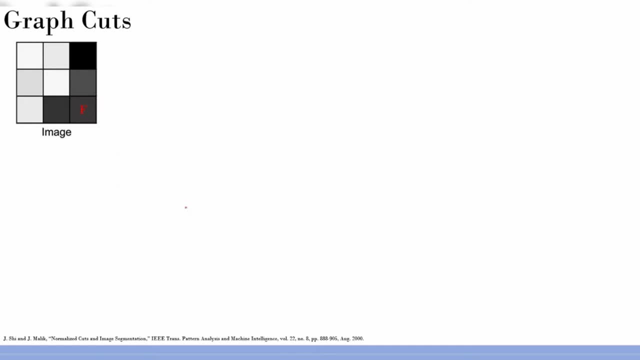 for us, ok, So let's start with that as we go careful. The idea is that let us do the following and we first step. we convert it into a graph. okay, so all these white pixels are considered as the background, okay, and the black pixels is considered as the foreground. so there will be a source. 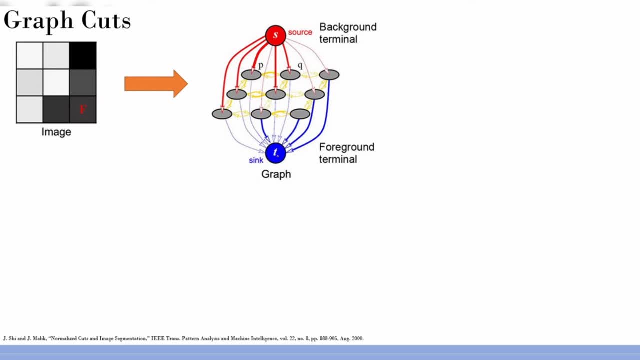 and there will be a target in the case, or sink in the case of a graph, and you can see the direction already. it will be going from source to sink all the time, and then each of these pixels are represented by these knots over here. okay, so there will be a super node, in fact, two super 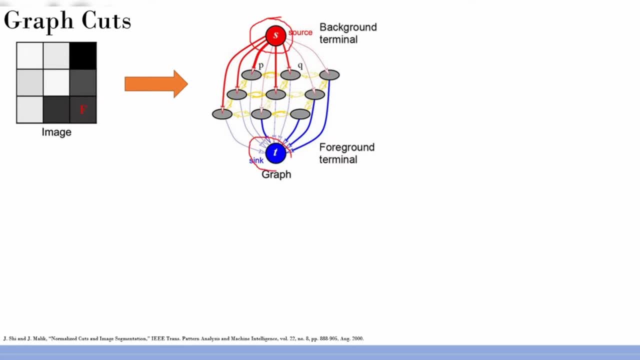 knots, one corresponding to the background, the other corresponding to the uh foreground. okay, so that's the concept. and then everything in the image, all the pixels are considered individually as knots. okay, so now this connectivity you see over here, you can see it's bi-directional, okay. 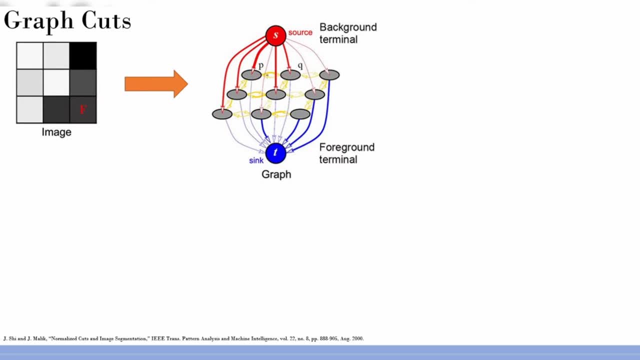 and you see the intensity also. so this, this weight, will be actually governed by the intensity relation between these two. okay, so that's a concept, and then each one will be connected. each of these pixels will be connected to the source or the foreground and the background. okay, and 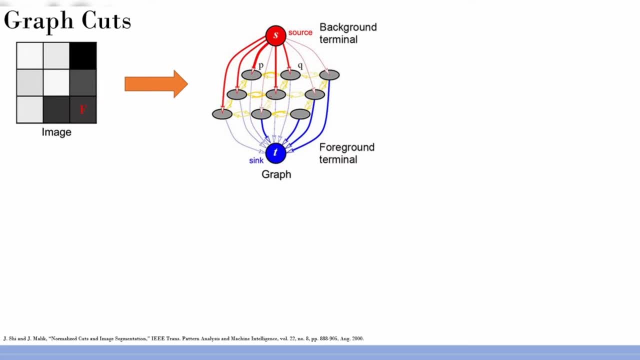 they will also carry a weight and i will explain how. how does it really work out? how does this weights? because other weight is easy, because it could be all these weights, right, all these weights. how does it work out? maybe i'll explain it in a very simple fashion. so graph cut is an. 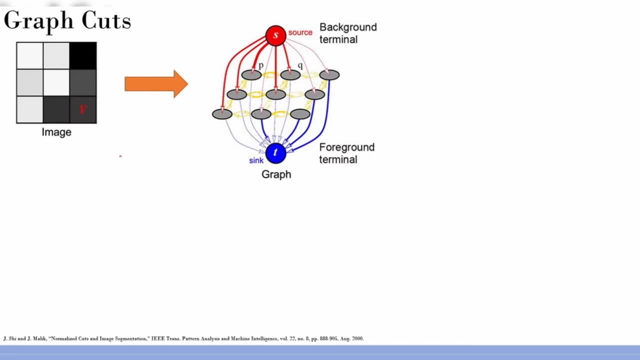 algorithm, which is an interactive segmentation algorithm. that means user is given the choice to mark some region as foreground and some region as background. so i'll illustrate also using matlab toolbox, a very, very easier way. uh, so first step is obviously for a user is to on the image you mark the foreground and the background, so randomly you can choose anything. 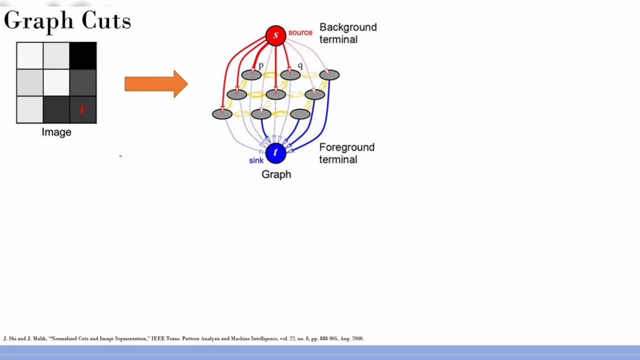 okay, and then those pixels are already given the weights because they are already marked by the user, so those pixels will be having very high weight to the source. okay, so those are the pixels which are already having very high weight to the uh source and the sorry foreground and the background. 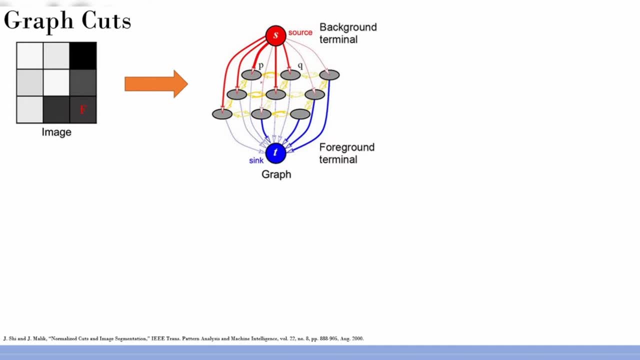 the remaining, of course, these, these weights. it's easy for you to calculate because it is some measure of the intensity and the distance measure between the pixels. okay, so i will explain to that at some point soon, so let's not discuss too much on that. so, once we make this graph, the next step. 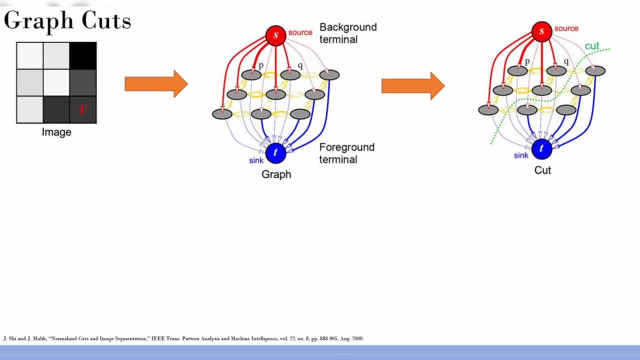 is actually to use graph theoretical approaches and to cut this graph into two. okay, so you do a cut and that cut is uh. cut can be based on various criteria and one of the most common criteria that people follow is max flow by the distance measure. okay, so you can use this graph to measure the. 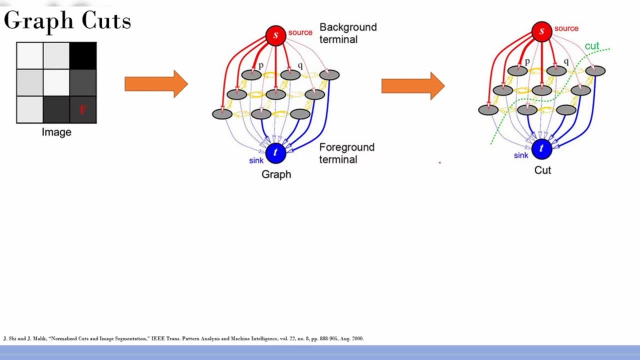 flow mean cut algorithm. it's a very famous algorithm in graph theory. i have an illustrative example, so with that i will explain to you what is it. so the idea is again reiterating: you convert the image segmentation problem into a graph problem, so you take the pixels as knots and 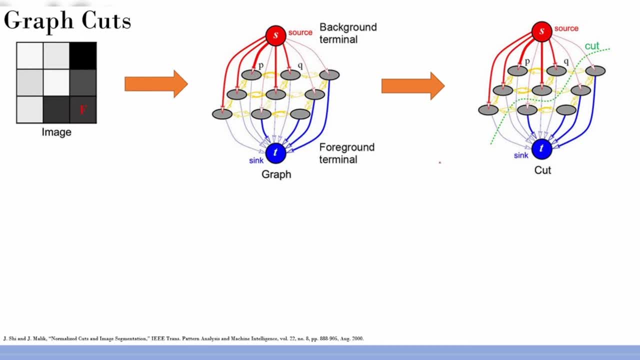 vertices. you ask the user to scribble on the image to mark as background and the foreground pixels and, based on those scribbling, you will create the entire graph using the super knots, also because the this part is quite straightforward for you. this, this part is quite straightforward forward for you. but the source to sync connection is uh, based on the. 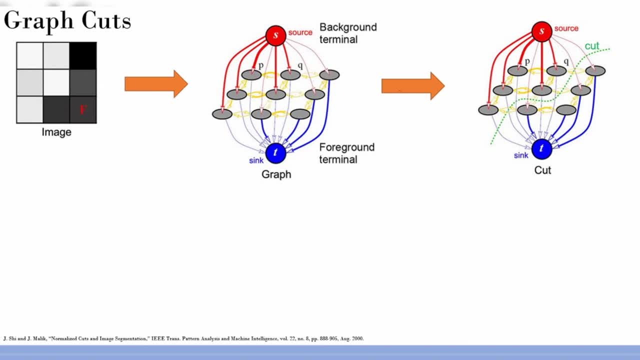 choice by the user. okay, and once we make this graph, we use graph optimization algorithms to have a cut. okay, the cut of the graph into two part, one belonging to the source or the background, other belonging to the uh, sync or target or the foreground. okay, the moment you do that. 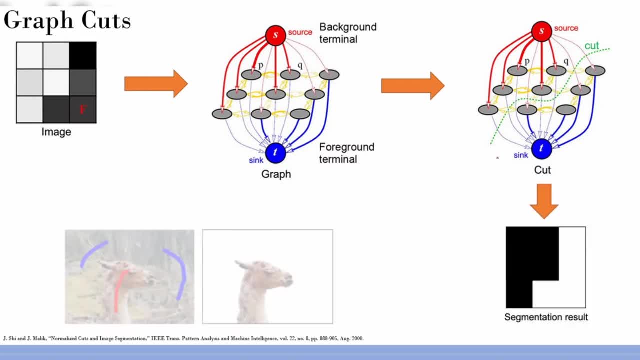 segmentation is done, that's it okay. so i'll have an example here. so this is what i was telling. so you have an image. i want to basically make a graph, and then i will make a graph and then i will make a separate this animal out from the background. so what we ask, first step is basically: you ask the. 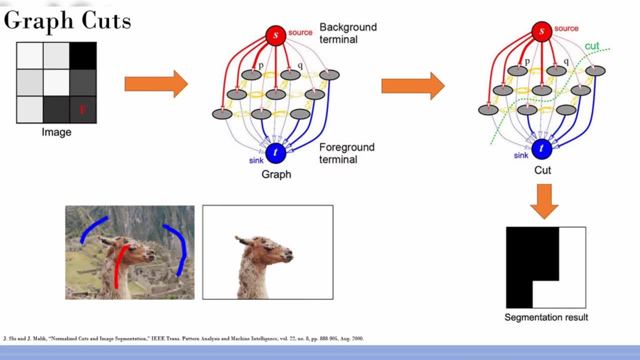 user to scribble the background and the foreground. so the choice is given to the user. so he scribbled this blue shade as the background. so two regions are selected, so these pixels immediately has the highest weight. okay, so sort of infinite weight which towards the- uh, let's say, this is the 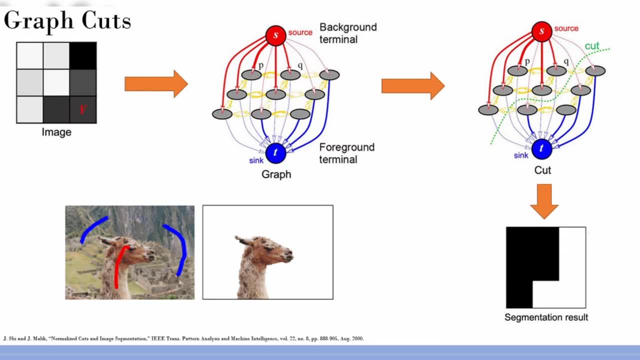 background right, and then this one is the foreground. so the red color, all these pixels which are lying in this line scribbled by the user, will be having infinite weight associated with the foreground. and then what our job is actually to find out for remaining pixels. okay, that's a very beautiful, uh thing. we will discuss that. so, based on some probability, 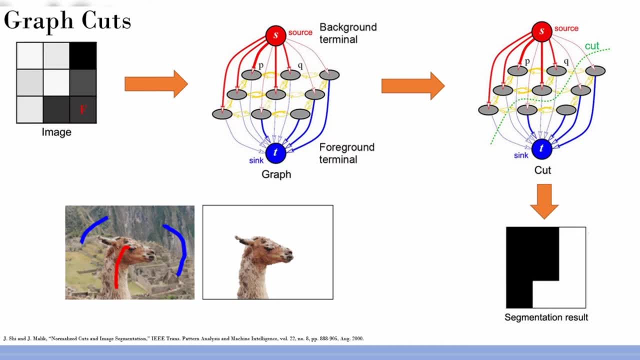 distribution. okay, we will actually decide the weights of those uh remaining pixels which are not really scribbled by the user. and then, of course, you do the graph cut algorithm, uh, or the optimization algorithm in the graph, to how the final result, and the final result looks like this: 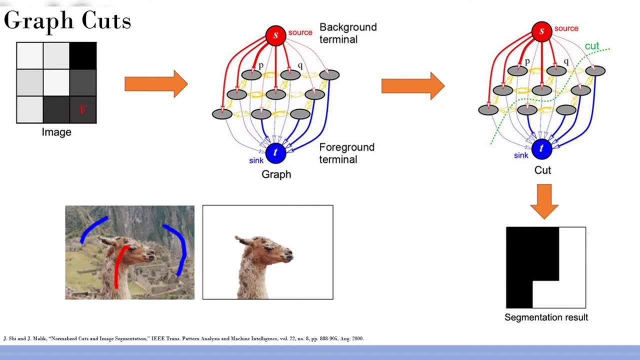 so, before going to the details of the algorithm, let me quickly show you the matlab example. okay, and of course python also opens you. we also ask the graph cut, so you can use that as well. but matlab i choose because it's very easy, it's a gui. 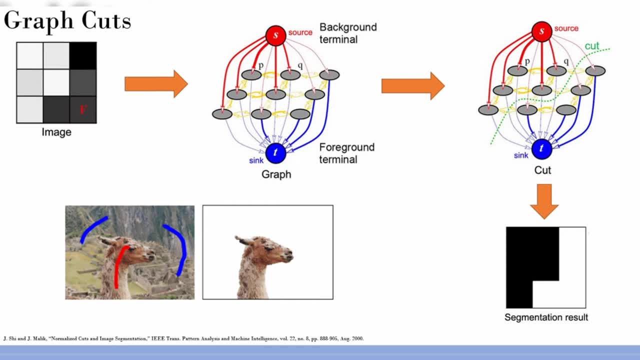 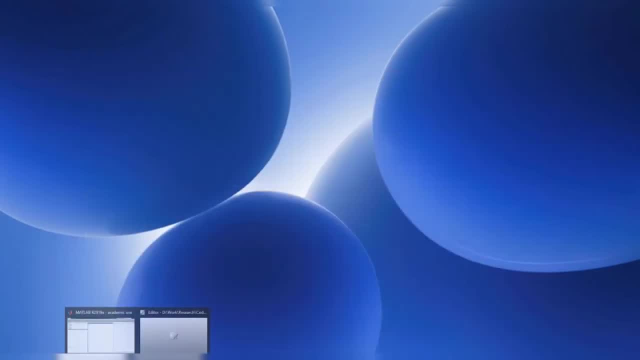 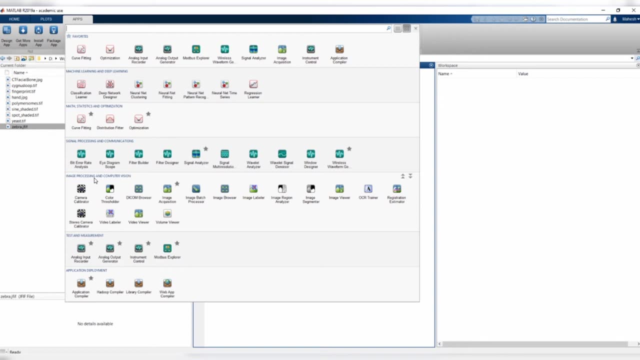 environment and it will very, very uh striking for you to be uh understanding it much better. so let me go to the matlab environment. okay, okay. so here it is. so if you go to the uh apps and then, of course, uh, you go to uh, if you expand it under the image processing, there will be a 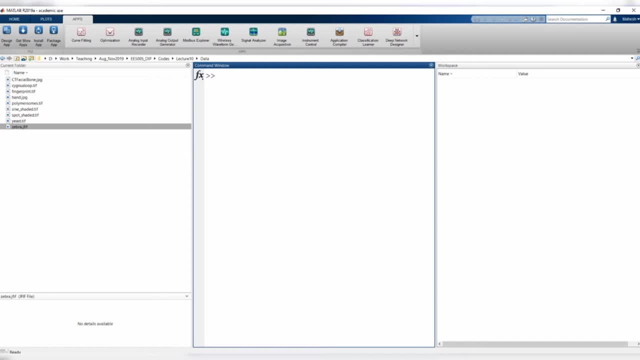 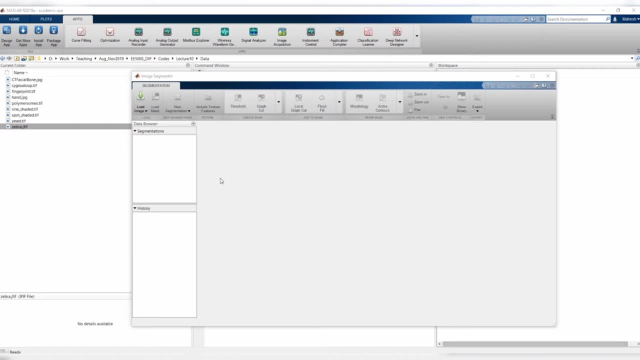 segmentation: image segmenter. you click on that so it will come. okay, so the window has come. it will take some time, depending on your processor, and then this is the window. so, in fact, this is a common image segmentation gui app for matlab. you can do all sorts of segmentation in this, but let's 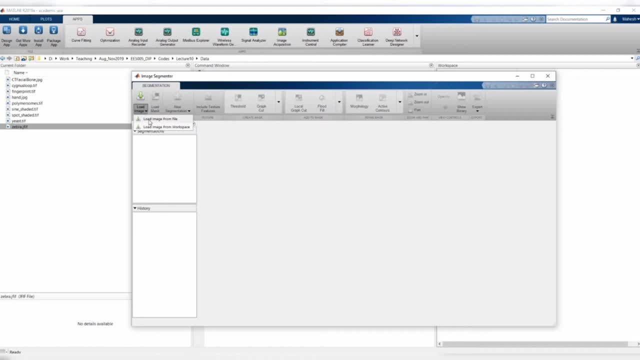 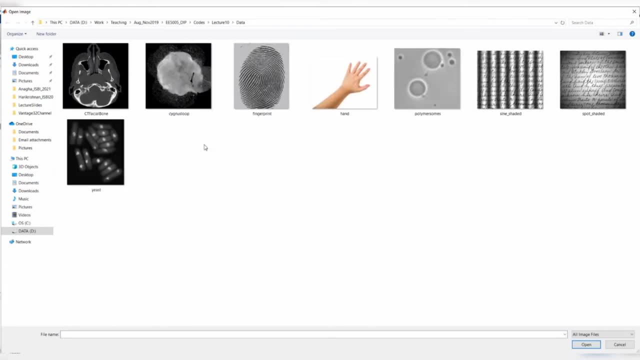 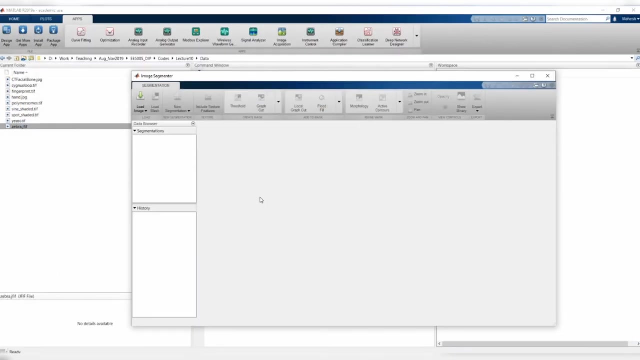 actually, uh, only explain um graph cut so you can load the image. so let me load one interesting image. uh, let me see. okay, you see, just view it. and uh, yeah, uh, yeah, let's put hand first. okay, so it's easier image to do, right, so i just took the hand. 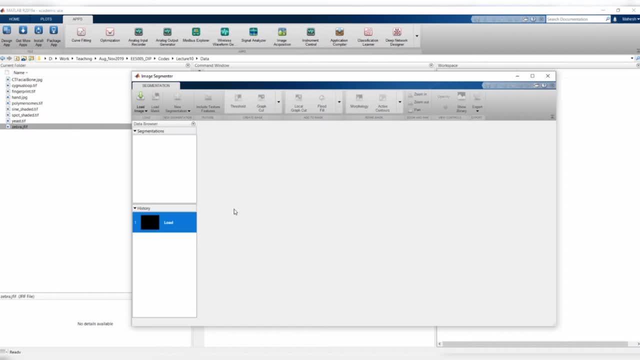 image and it will take some time to load. okay, so the image has come. now i choose graph cut. okay, so you can. actually the auto cluster is nothing, but the k means okay and circles is half transform, or if you remember. so let me put the graph threshold. sorry, graph cut algorithm here. 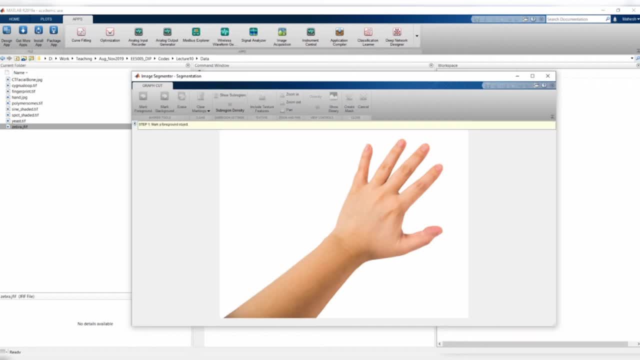 i choose in the graph cut. so it takes some time and then you have, you're seeing, here on the top. you can mark the for uh foreground and mark the background. so let me just put: foreground is here. here you can scribble as many you want and then you choose background and 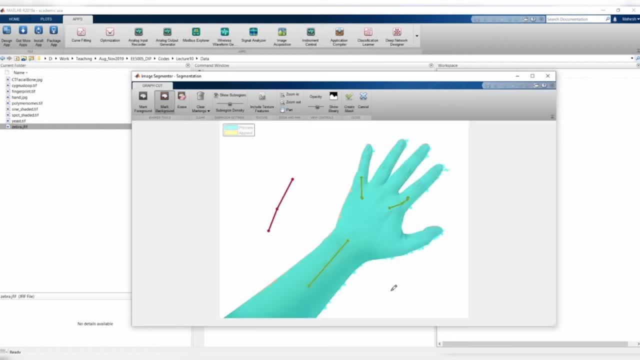 this is easier. actually, this image is quite easy. you already see the image is segmented. that's it. so, uh, the the beautiful, beautiful, uh thing about this is you moment you scribble the background foreground. the algorithm is working at the back end and it is already segmented. the thing out right and now. 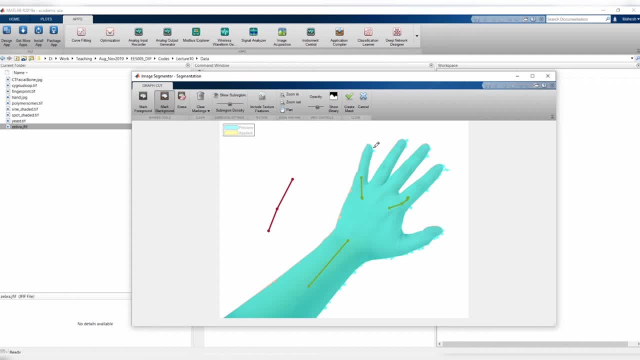 the view. this is an interactive so i can actually choose, uh, some of these wrongly uh region if i see, oh, that's over segmented, so let me just run, okay, so you can see it. so there's some uh problem here which you can correct it if you want. and then one more thing i just quickly wanted to show you is 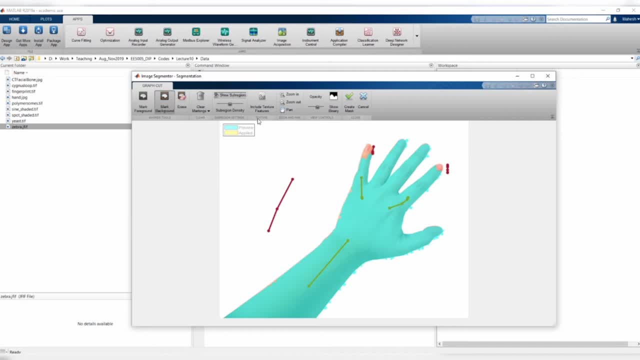 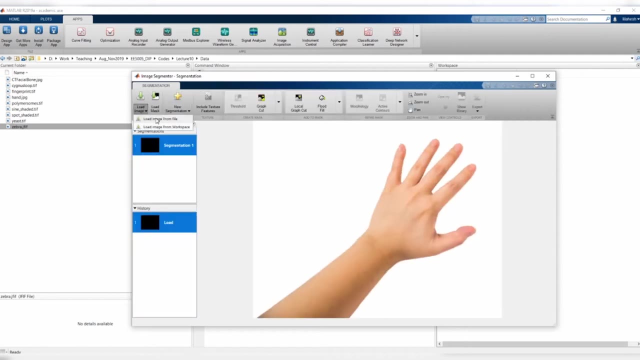 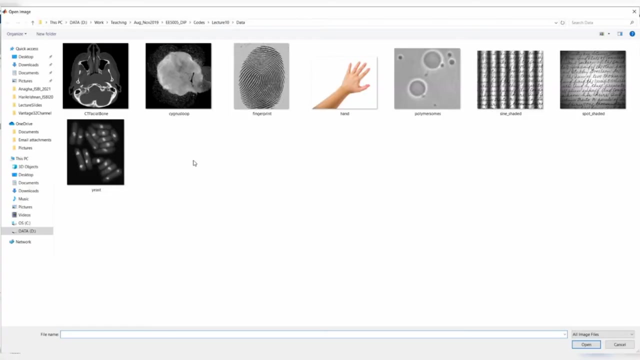 this uh, show sub regions option, which is sort of super pixel that we were talking about. so this background it uses super pixels well, so just wanted to show you that. okay, and uh, let me take another example. so let me just cancel this. uh, load another image. uh, in this case, uh, let me just take. i think you should have more. 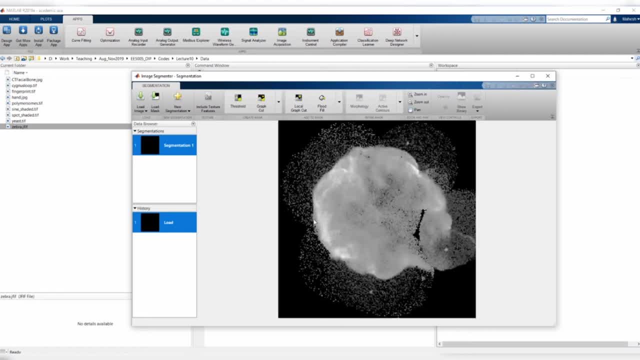 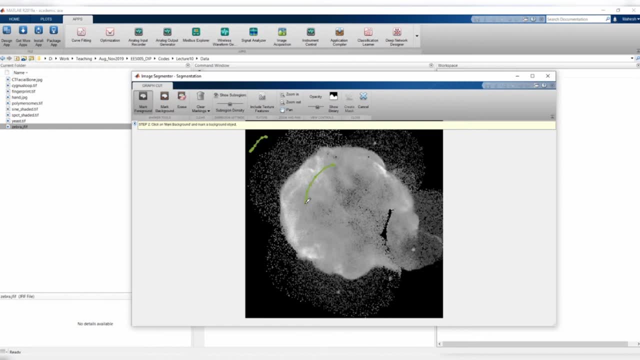 interesting images. okay, so this is chosen. now let me do graph cut again, so i will choose the background. so let me choose this one as the background, this one the bag. I just want the similar problem that we were facing earlier. right, so as many as I want. 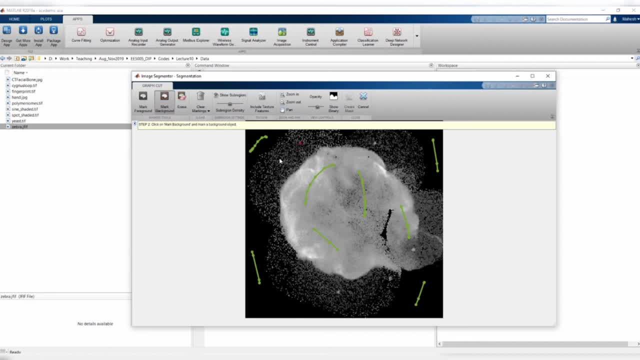 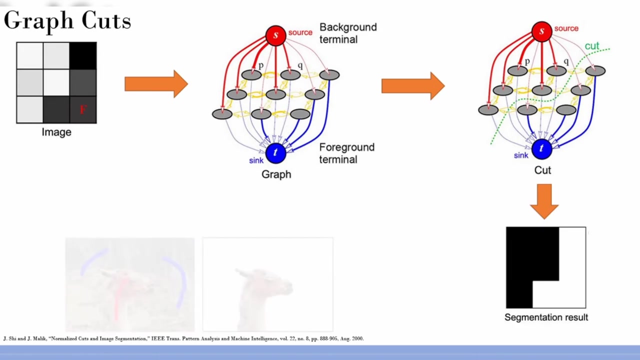 okay, now let me put the background so I can in fact choose. okay, so sort of, I got everything right. so this is the beautiful concept of graph cuts. now let me go back to the slides and explain what we did. okay, so that's it. so I hope this part is clear to. 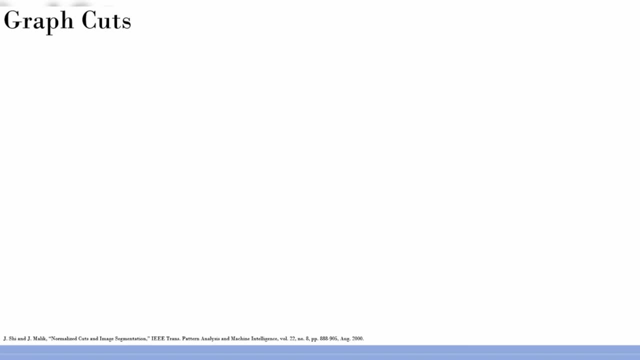 you. now. let's go to the algorithm in detail. what's happening? okay, so the first step is, as we explained, you construct the graph. okay, so v stands for vertex and e stands for the edges. so you here. in our case, we will have basically all the pixels in the image as the nodes, and then we will have a. 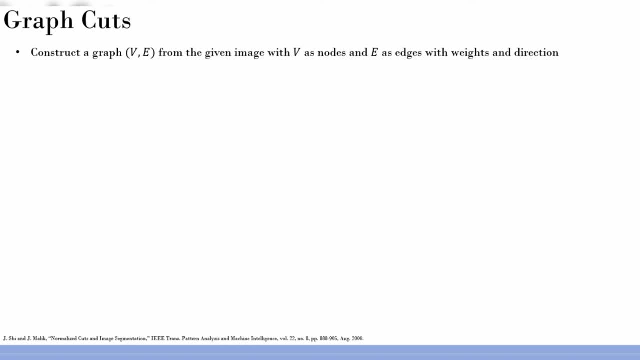 super node for the image, and then we will have a super node for the image, and then we will have the background and the foreground, which is governed by the scribbles from the user. okay, so the graph will have a direction also and the weight also. so the weights, let's say with this is: 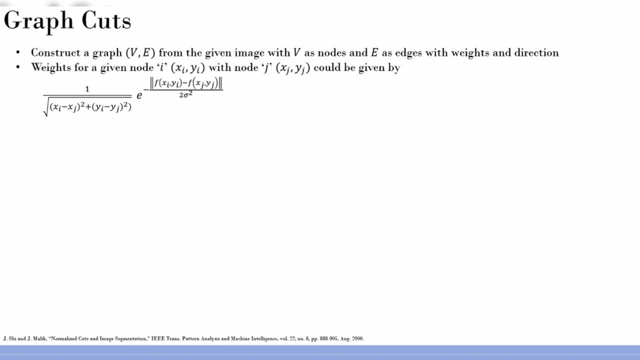 I am not talking about the connection from the super node, or the background, or the foreground, to the pixels, this interconnectivity I am talking about. so, between pixels we can have a weight given by, let's say, from node i, which is nothing but one pixel, to other pixels, so pixel i to pixel j. 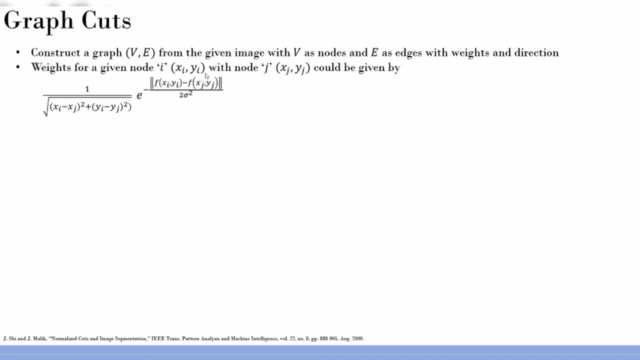 okay, so let the location be the same, so we can have a weight given by, let's say, from node i. okay, so let the location of those pixels be x, i, y, i and x, j, y, j. if that is a case, it is given by a very simple formula here. okay, so this is the normalization by distance. okay, so you normalize. 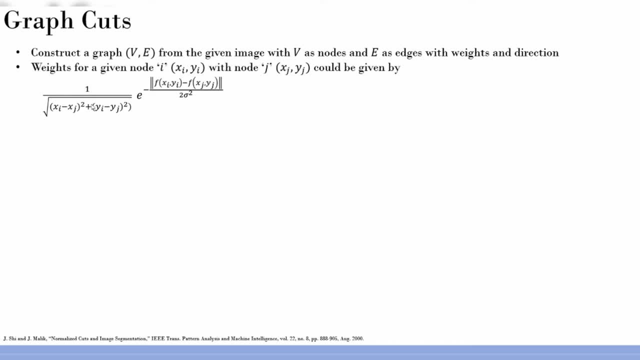 by the distance, because you should have some weight to the distance as well, right? if it is quite far away, it should have a lower weight, right? so that's a concept here. so euclidean distance here, and then this is nothing but the intensity difference, square intensity difference. 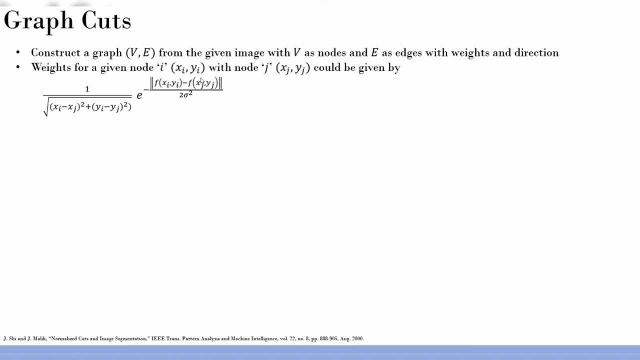 so x, i, y, i intensity at that pixel, minus x, j, y, j intensity at that pixel. so this is the pixel square root of that, right, I mean square and square root of that. so, and you can give a factor of sigma some variance also if you want to keep so. let's consider this: suppose the pixels 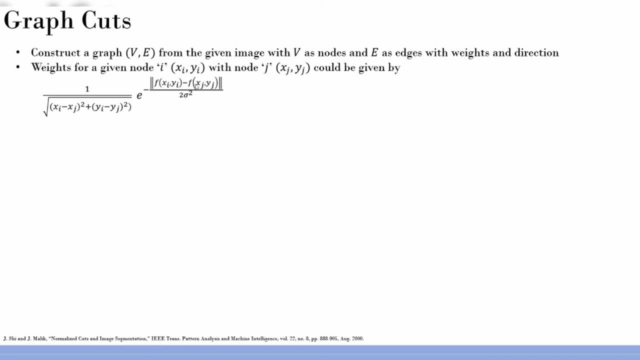 are having very cross intensity. so f of x, i, y, i is almost equal to f of if. if let's say this condition- I am sorry, this condition is what I am talking about- okay, so let's say f of x, i, y, i is nearly equal to, let's say, f of x, j. 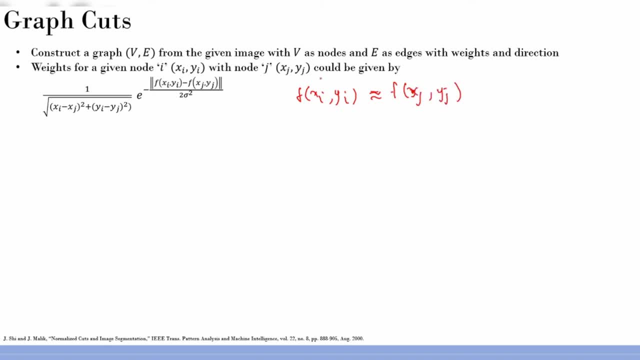 y, j. okay, so if that is the case, that means this: this guy will almost go to 0, sorry, 0. so then e, raised to 0, will almost goes to 1, right, so that's the concept. so this, this entire term, will become 1 and it is only weighted by the distance. now, if, in other case, if there is a huge difference, 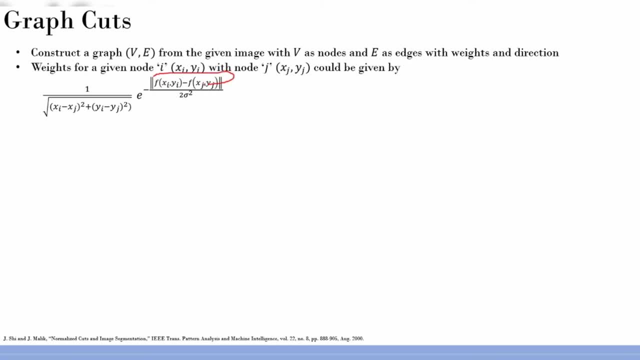 between these two. if this is a huge difference, this value increases, this value is going to increase and we already know that if this value is going to increase, this entire exponential will tend to be closer to 0. so that means if there is good connect, good intensity relation between the pixels, they 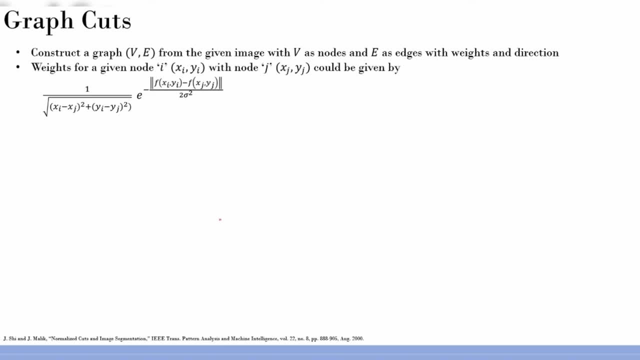 will be given higher weight. if the intensity difference increases, then the weight will be actually going down almost to 0. that's what you want, right? I mean it's satisfied. so this is how you can you create the connectivity between the pixels or within the image region. okay, 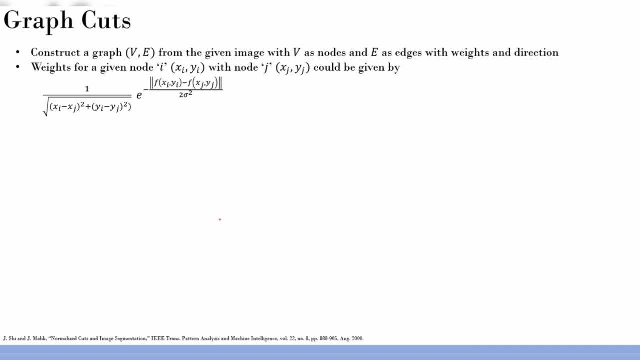 and then, of course, if two pixels are having same intensity but they are far apart, they should be given lower weight, and that will be taken care by this guy over here. okay, so that I'm. I hope everyone is clear with that aspect. so this is what we actually do. I'm just go back and show you what. 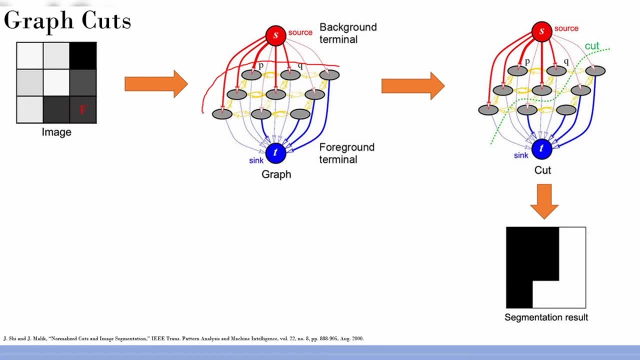 exactly. I meant this is for this particular thing. what we are talking about is this connectivity alone. we never talked about this connectivity- how to connect to the background and the foreground. okay, so that's what we completed. now let me go back again. okay, so that's done. so that's a first. 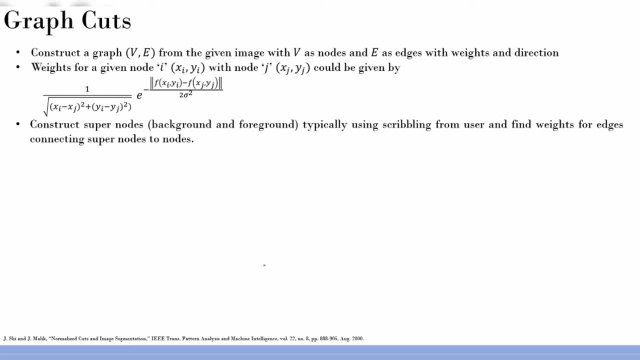 step and then we create the super nodes background and foreground. so this is done by asking the user, just like we saw it in matlab. right, you are asked to scribble the background and the foreground. so once you scribble, it's a very interesting. so of course, those pixels which are scribbled are already known to you. so for 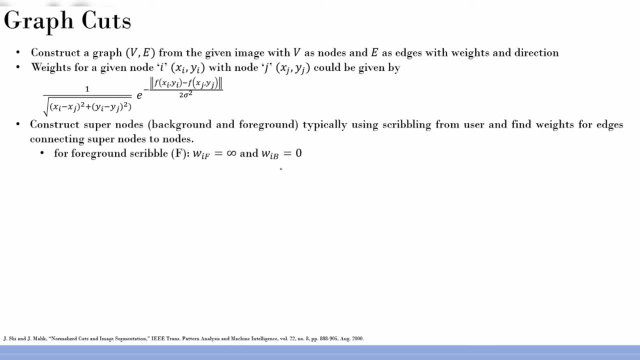 foreground scribble. so those pixels which belong to the foreground you have to give infinite weight right, because you are 100 percent sure that is belonging to the foreground and then the background. in that case the what I'm talking about is the connectivity. let's say one pixel. 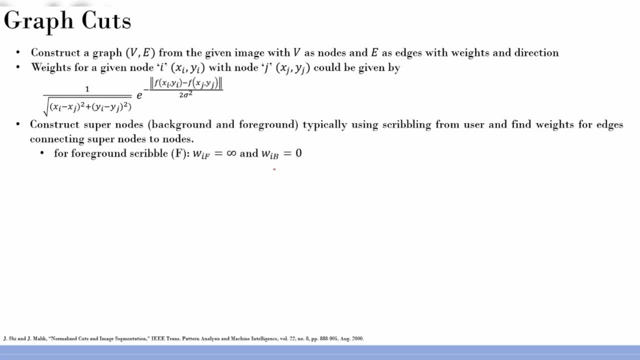 you are already scribbled it as a foreground script- I mean you already marked it as a foreground pixel- then the connectivity of that pixel to the foreground should be infinity and to the background is zero, because you already make sure that is a foreground pixel. okay, so that's what I'm. 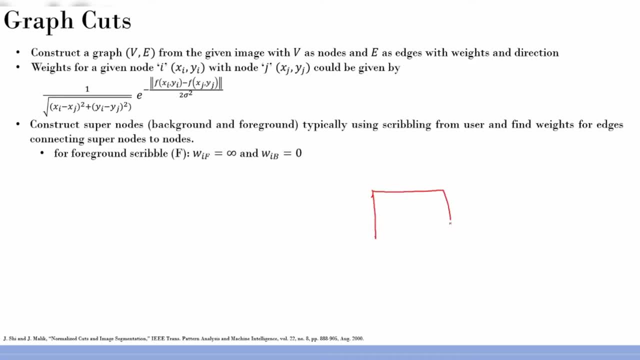 talking about. maybe pictorial representation may be better. so this is the pixel image here. this is your background and this is your foreground. let's say: okay, so this pixel. let's say this pixel. I already made sure this belongs to the background. so this is background and this is foreground. ok, foreground node. 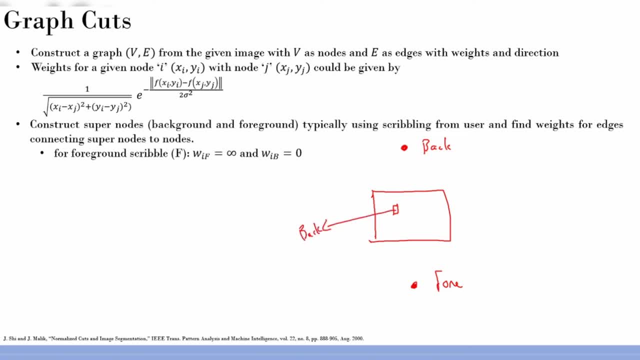 So this, I am marking it as background, scribbled as background. so then there is a connectivity like this. let us say: ok, So this connectivity will be wif will be infinity, because it is sorry, wib in this case. and then this connectivity to the foreground, wif is equal to 0 because I marked this scribble. 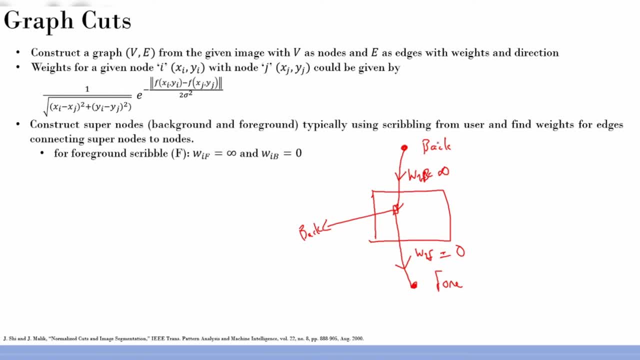 as background, So it has to be infinite. it has highest weight and, connected to the background and foreground, it should be 0. So it is simple, right? I hope I am not confusing you So, because those are the pixels marked by the user and similarly for the background. 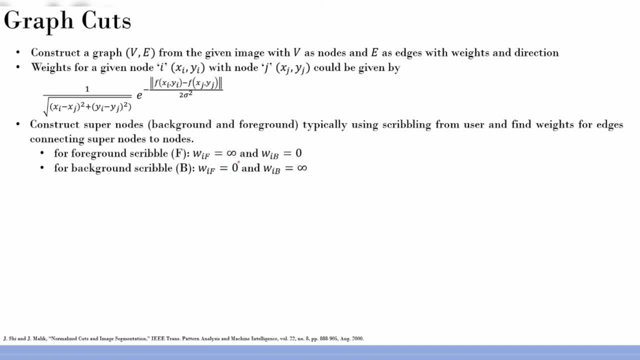 it is opposite right, so that if that pixel belongs to the background, then of course it should not have any weight with the foreground. it should be having infinite weight with the background because it is a background scribble. ok, so that is it. So this is also done. 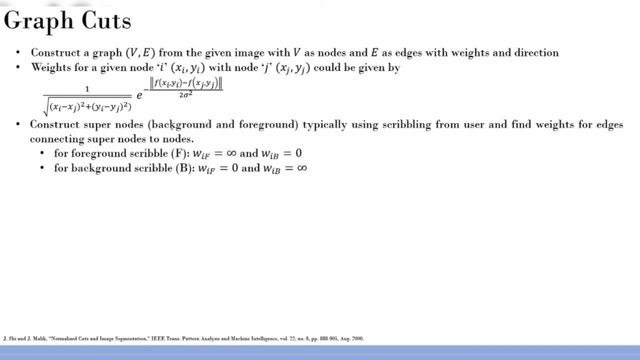 So you started with the pixels to pixel connection. you have a weight. the edge weights are given by this equation. then you ask the user to scribble the background and foreground and those pixels which are scribbled by the user. you will have either infinite weight or zero. 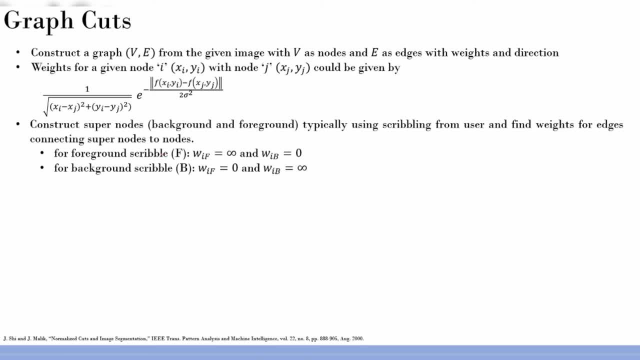 weight with the corresponding node. right, If it is a foreground scribble, you have infinite weight with the foreground node, zero weight with the background. If it is a background scribble, you have zero weight with the foreground and infinite weight with the background. Now what about remaining pixels? those pixels also have to be connected to the foreground. 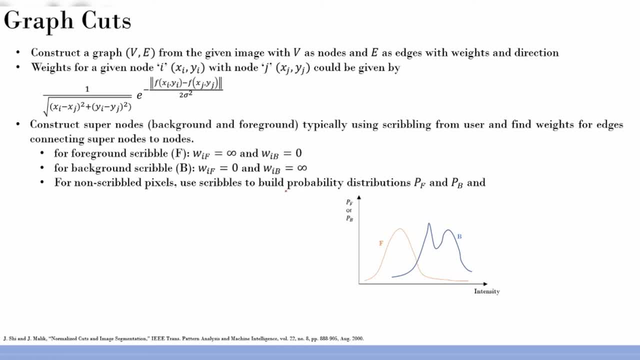 and background, and that is where the beautiful concept for non scribbled pixels use scribbles to build the probability distribution. So what we do is You have so many pixels which are marked as the background right and you have so many pixels which are scribbled by the user as the foreground. 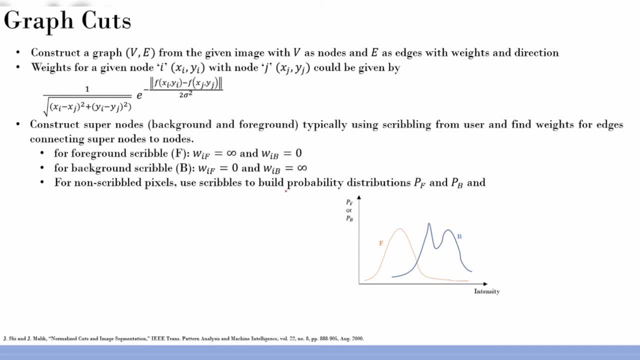 You create an intensity, a probability, that histogram, basically nothing much, the normalized histogram you could call So the normal. let's say I scribbled so many pixels, some number of pixels, as foreground, and if I plot the histogram, this is how I get, let's say, some example. ok, 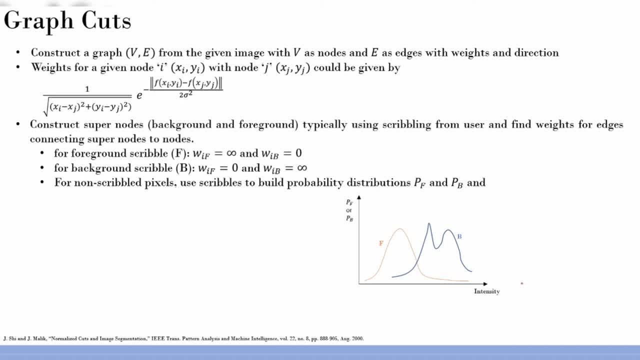 So this is the distribution. the orange color is the distribution I get. so x axis is the intensity, y axis is the normalized histogram count. ok, So this is the distribution for the foreground, ok. And similarly, if I take histogram for the normalized histogram for the background pixels: 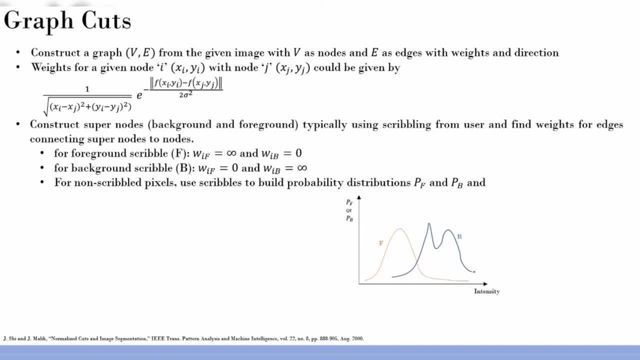 which are scribbled by the user. I may get a distribution. Just this for illustration. any shape it can take, ok, Now comes the beautiful concept. ok, Now let's say I have a non scribbled pixel. ok, Some non scribbled pixel which was not scribbled by the user somewhere in the outside region. 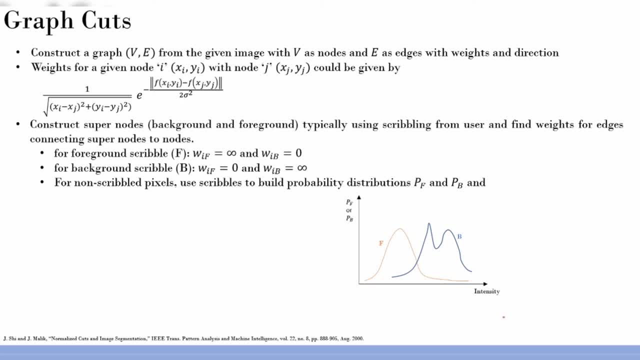 of scribble. So you take that pixel, you consider the intensity of that pixel. Let's say that intensity is coming somewhere here. ok, So this is the intensity of that particular pixel which is non scribbled by the user. Now this: if I see this intensity, there are two values associated with it, right? 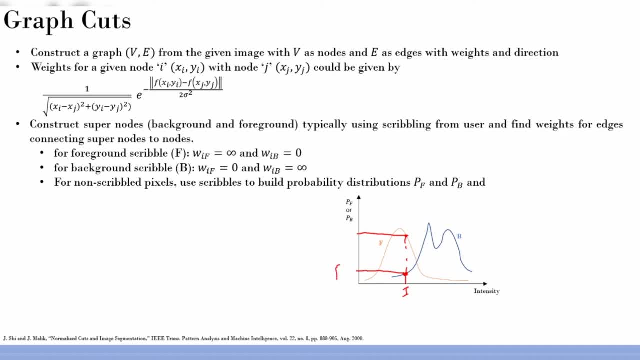 So this value which is actually lying on the curve is pb and this value which is lying on the histogram of f is pf. ok, So this essentially means that this pixel, This pixel, has a probability of pf to be belonging to the foreground pixel and pb to be belonging. 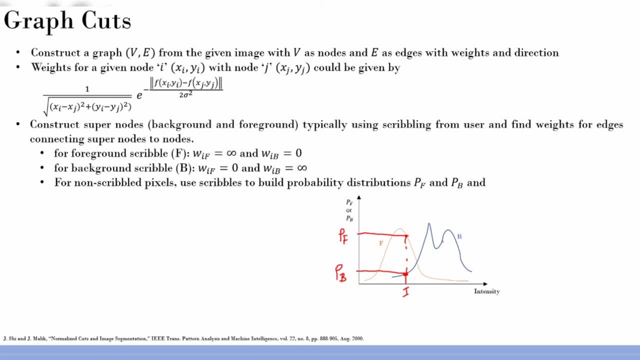 to the background pixel. So that's the concept, ok, So moment you have that. ok, So what you do then is basically use this expression ok to find out the corresponding weight. ok, Let's actually see in this case. In this case, pf value is going to be very high, right? 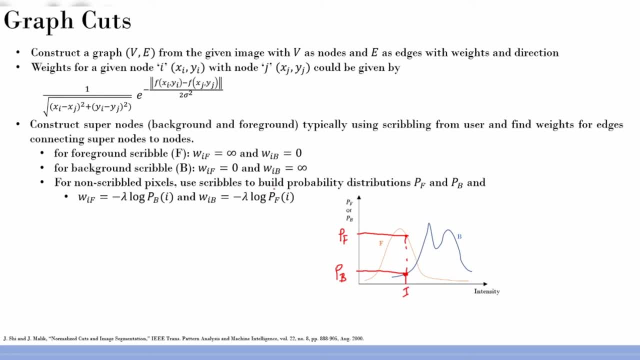 In this case, pf value is going to be very high. So I put pf value. It is going to increase. So if the pf value is going to increase, ok, If this is going to increase, that means this log itself is going to increase and minus. 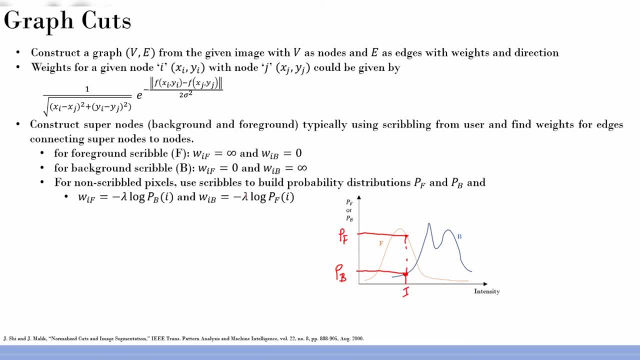 of this. lambda is a hyper parameter. you can put some regularization, So otherwise this value is going to be negative, right? It is going to be like really, really high value, right? So that's the thing. So that means this: It is the chance that this pixel is. 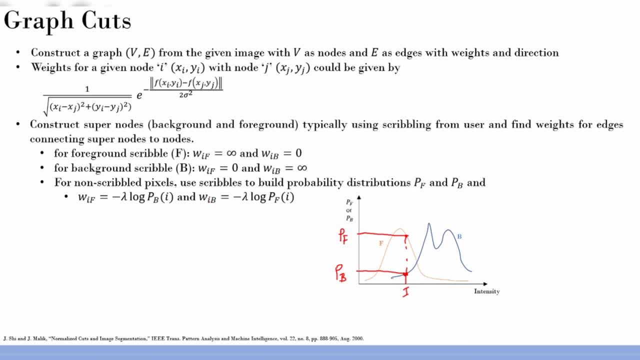 This weight is really low And in this case, for example, the pb value is going to be very low, So this value is going to be very low. That means this is really going to be negative. Log will be going. Log of small value will be negative. 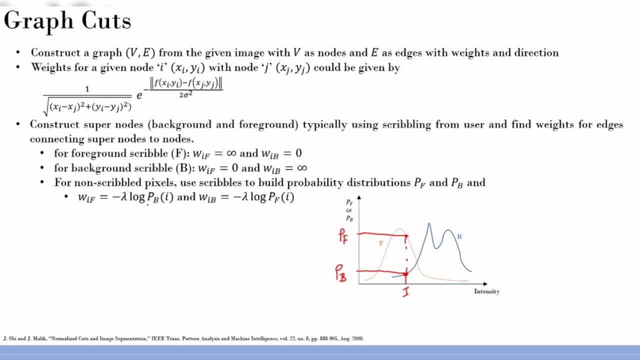 And this negative sign will make it positive And it goes to almost like low value. That means this is going to increase. So that's what essentially happens here. So this It is sort of inverse relation, Because if has a probability, pb here 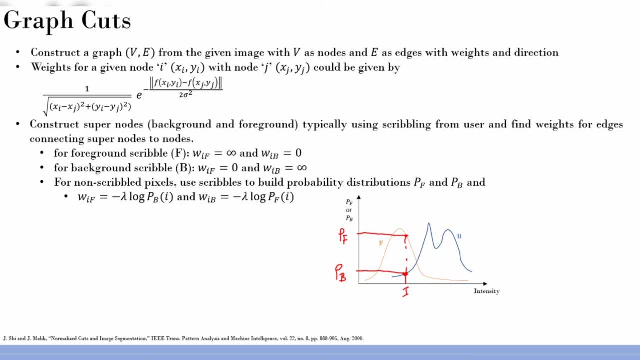 And ib has a probability pf here. So basically, high value of this will make it more negative This guy to be more negative And low value of this will make this guy to be positive. So in this particular example, pb value is quite high. 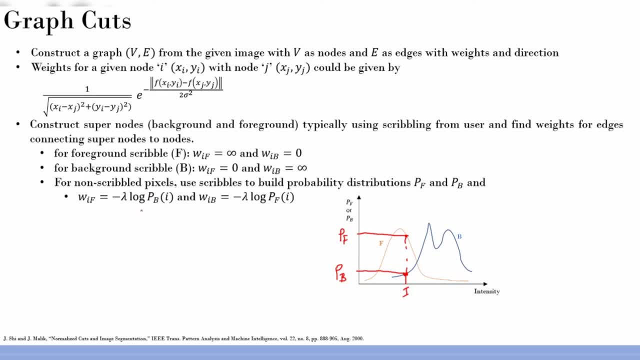 That means Sorry. pb value is quite low. That means this value will be sort of negative And then this negative term will make it positive. Pf value is very high. That means this particular thing will be positive. Y negative value makes it negative. 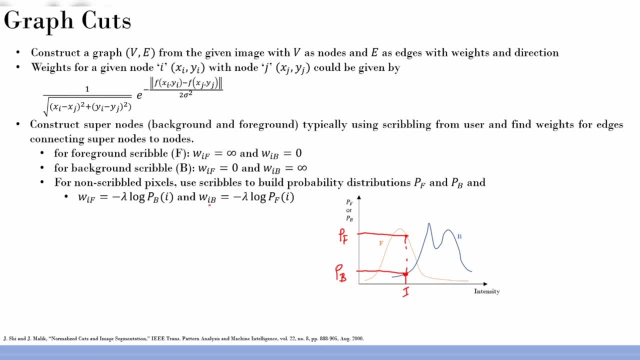 So that means The graph is really having that weight automatically. You don't really have to worry. So let me just reiterate again what we did. We considered the image. Then first step we actually did is we consider each pixel in the image as a node. 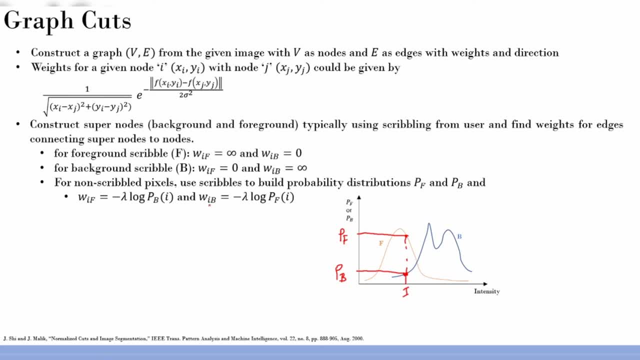 And then the next step is to find the weight of the edges, which is actually connecting this particular pixel to all other pixels. For that you use this particular formula. I hope this is clear to you. After that, the user is asked to scribble the background and the foreground to create the. 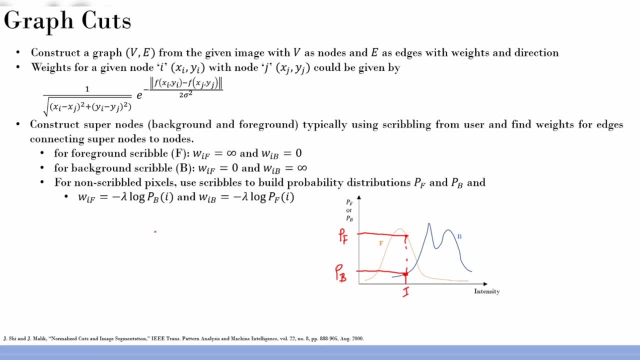 super nodes, Right. So when the user does that, the thing is like: all those pixels which are scribbled by the user will be automatically given infinity or zero weights. There's no problem there. And then non scribbled pixels: you go to the. you go, you create the probability distribution. 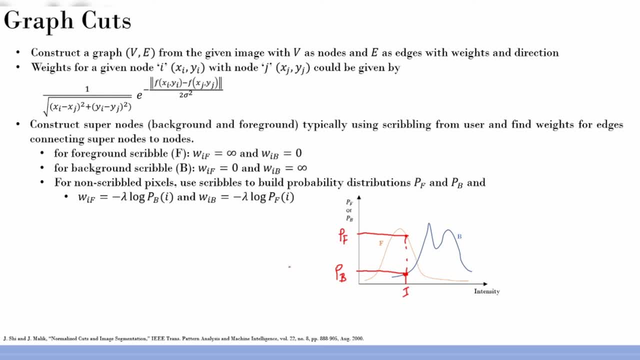 from the scribbled pixels And, based on this probability distribution, you go to each and every non scribbled pixel. You see the pf and pb value from these plots And then use this formula to actually assign the weights. I hope it's very clear. 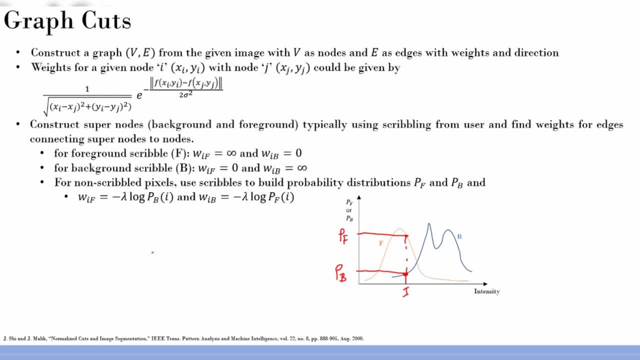 There is no chance of confusion here. It's a. It's an interesting and very easy approach. The moment you have that, you made the graph right, You have all the nodes ready, all the connectivity ready, and then you converted the image segmentation problem into a graph problem and now you can go ahead with solving it using all classical. 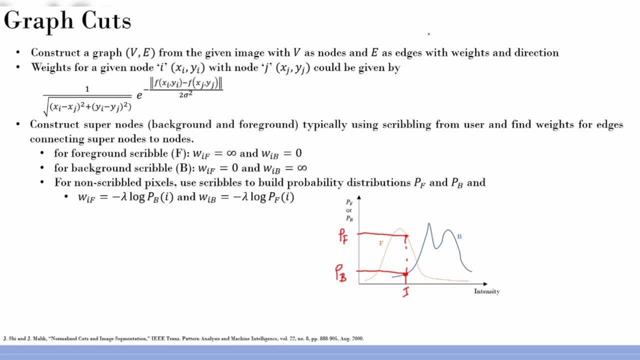 graph algorithms. I mean lot of algorithms are available, So that's it. Let me just discard this marking. Okay, so then I will relay on well established graph theoretical concepts. One of the concepts which I'm going to explain to you is max flow, min cut algorithm. 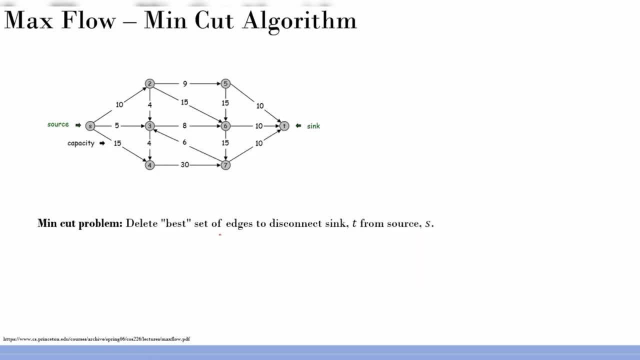 Okay, so let's take a look at that algorithm. Okay, so this is what I was telling. so convert your image into a graph like this: So your source is and source and sync will be actually the super nodes, which is scribbled by the user. 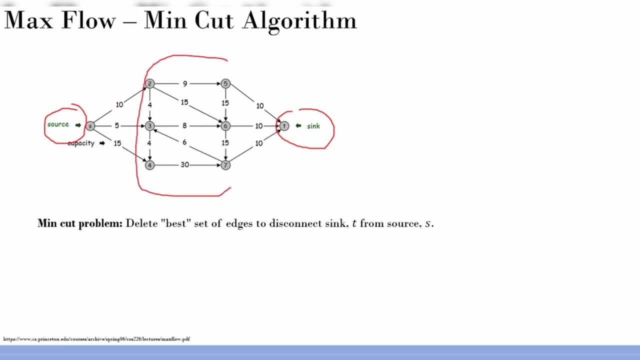 Okay, so always remember that. And then all this is your pixels, Okay, and each of. in this case, I'm not so showing the connectivity between this to this, Okay, So remember that. also, to every pixel, we have connectivity between the source and this one. 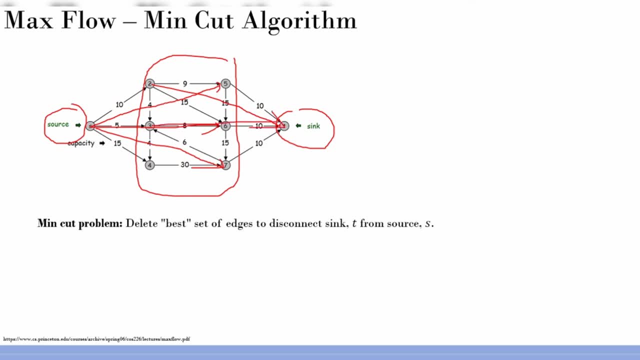 Similarly, this also has connectivity to here, So I'm not showing that for the sake of explanation, right? So always remember that. Okay, and the min cut problem: Okay. so we'll approach. I will explain to you what exactly happens. I hope it's clear how to convert the image to a graph. 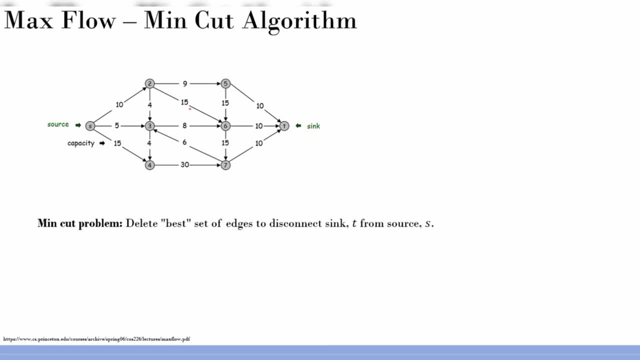 That part should be very clear. I think explained in the previous slide Moment. we have that. the result is a graph. Now we need to do is cut this graph into Some belonging to the source and one belonging to the sync. That's our target. 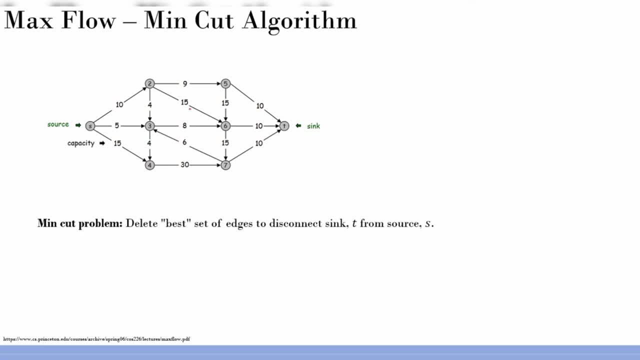 Okay, so one, two ways, two things we are trying to achieve. There's a min cut algorithm, which is very famous, And there is a max flow algorithm, which is also very famous, But the most robust algorithm which is used in image segmentation is something on us- max. 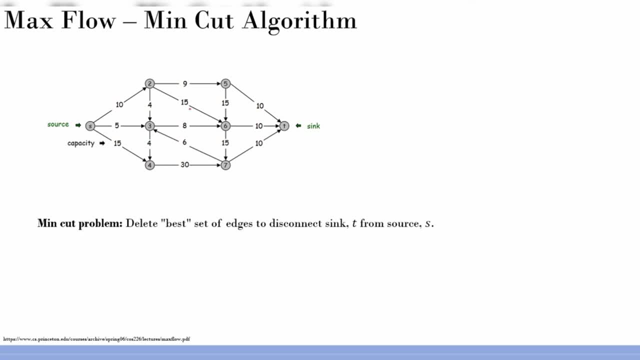 flow min cut algorithm. So we are going to discuss on that in detail. Okay, so let's start with the min cut problem. So delete the best cut of best set of edges to disconnect sync T from sync source. That's objective. Okay, and some definitions. I just wanted to reiterate that. super knots. 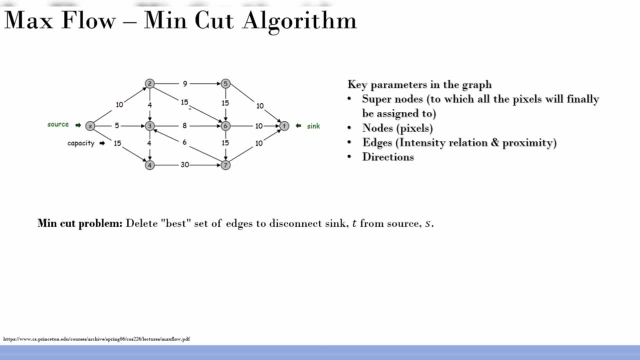 Okay, super knots are the pixels to which, finally, it will be assigned. it's our background and the foreground. Okay, so as simple as that. knots, all the pixels, all the pixels in the image are knots. So, including super knot, we will have, let's say, I have an image which is n by n in shape. 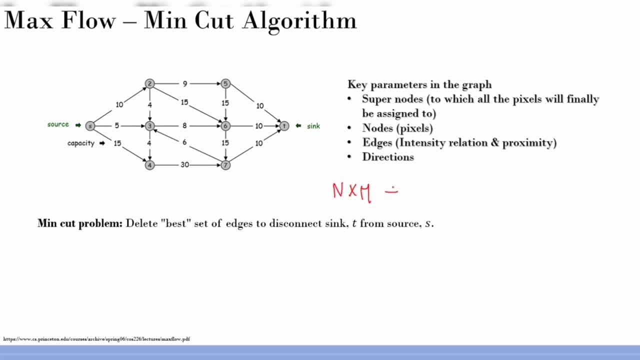 So total knots in the image is n, cross, m plus two super knots right, one for the background and one for the. So these are the number of knots, total number of knots in the image, and out of that two knots will be super knots, one for the background and one for the foreground. 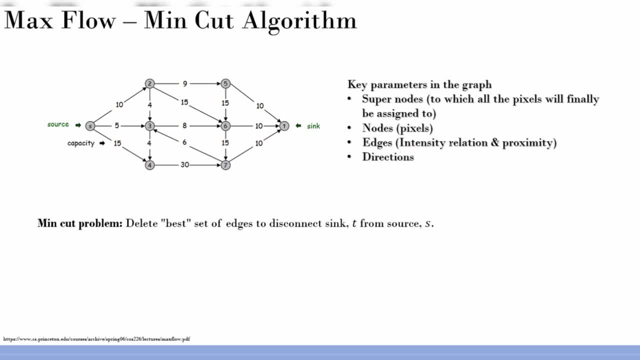 And then each of these knots are interconnected by edges, will have an intensity relation and, of course, the proximity also. right, wait, we already saw that direction also is there. Okay, so from source it will be always forward, from sync it will be always backward, And then, of course, between pixels, the direction can be governed by the distance or from the. 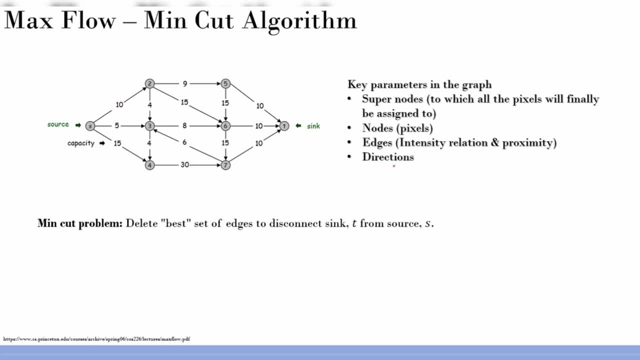 source to sync automatically. that negative sign will take care of, So you don't have to actually worry about. okay? So these are the concepts. I hope it's very clear to you. now let's start something very interesting. okay, So I'll take an example so you can go to this lecture if you're not understanding what I'm. 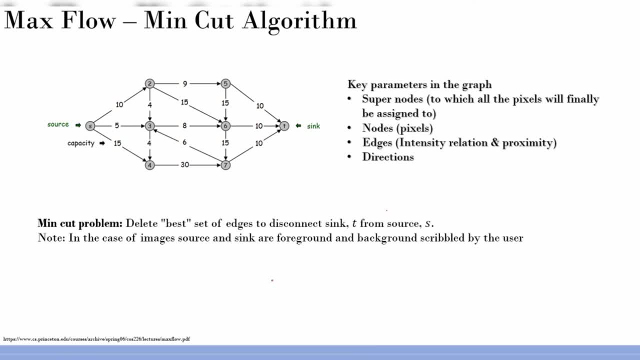 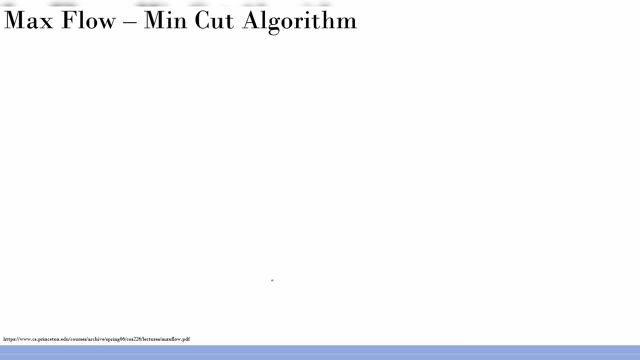 saying is explained beautifully here. also, I take I borrow from them. okay, This again reiterating: in the case of images, source and sync are the foreground and the background scribbled by the user. we already saw that in MATLAB. that's why I showed you. 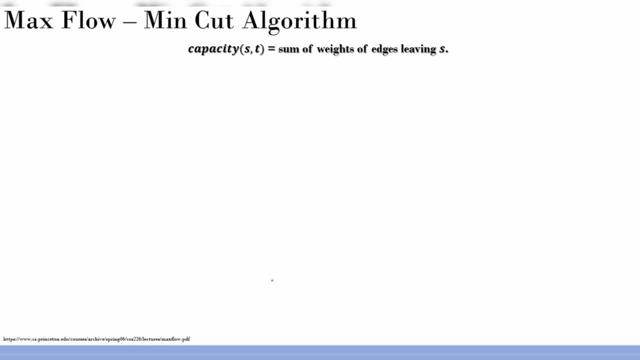 the demo. and then coming back to the explanation, Because always It gives you that in duty, you can imagine your mind right now. there are certain definitions in the graph. those who studied graph should be well aware of these definitions, but those who are not studied, I will explain to you in this slides. 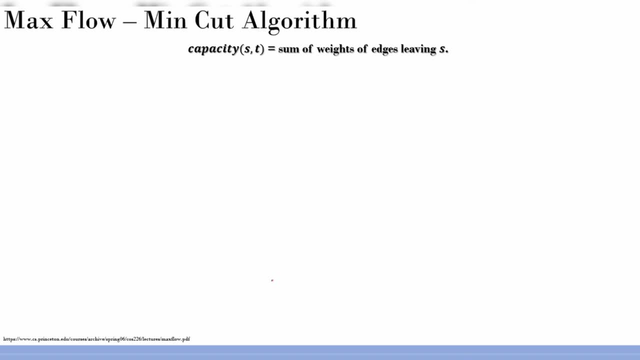 So capacity of a, basically a node, let's say, okay, a particular node, or I would say a capacity of a graph is basically the capacity from s to t source to sync. okay, is the sum of all the weights of edges leaving that particular node. Let me, let me. 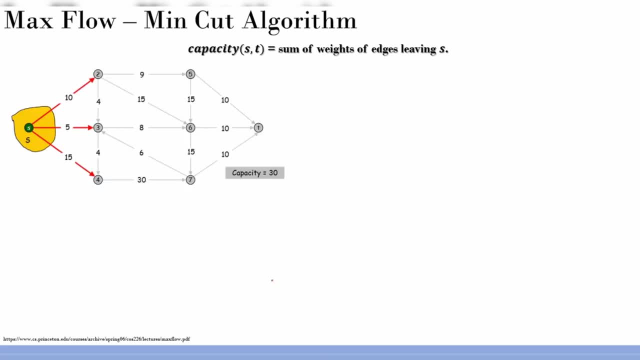 So source can be a node and target can be, or sync can be another node. So let's say one example I will, I'm going to take. So capacity for this guy s, this node s, is nothing but the sum of all these edges, okay, sum of all these weights, 10 plus 5 plus 15, 30, okay. so you have that okay. 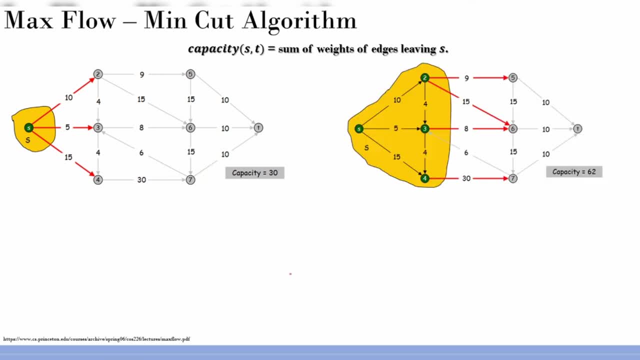 So I have some more examples so it becomes very clear Again, the capacity for this particular case, this, this particular thing. when I consider This is only considering this now, I am considering all these particular nodes. So if that is the case, this is the capacity, okay, 9 plus 15 plus 8 plus 30, which is 62.. 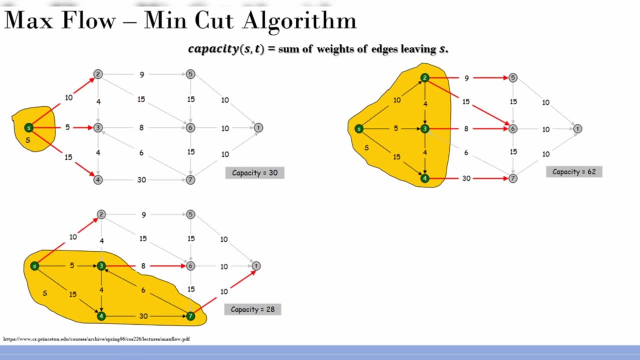 And similarly, for if I consider this set of nodes, the capacity is 10 plus 8 plus 15, which is 28. okay. And similarly, now min cut problem is find an s? t cut of minimum capacity. So in this case, of course, the minimum capacity I would choose is this guy, okay. 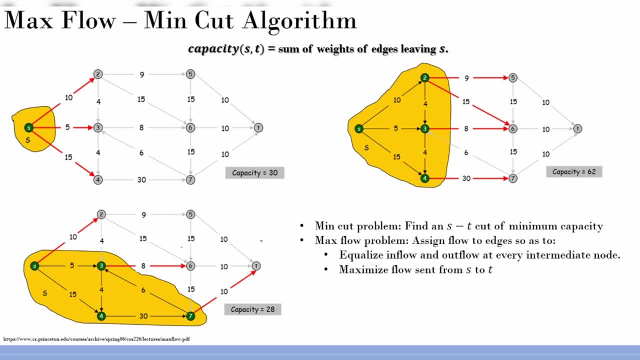 So that's the example. Now there is another. this: this may not always give you the optimum result, So people have proven that min cut will not alone. if you go for the minimum capacity alone will not give me the best result. People also consider this something known as flow. okay, 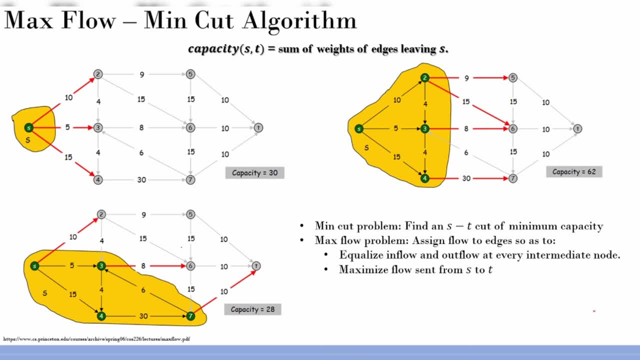 So what is flow? flow is basically something like you assign some flow to the edges. So this is a maximum capacity that can go from s to node number 2- 10. okay, So you can't go beyond 10, but you can vary between 0 and 10, okay. 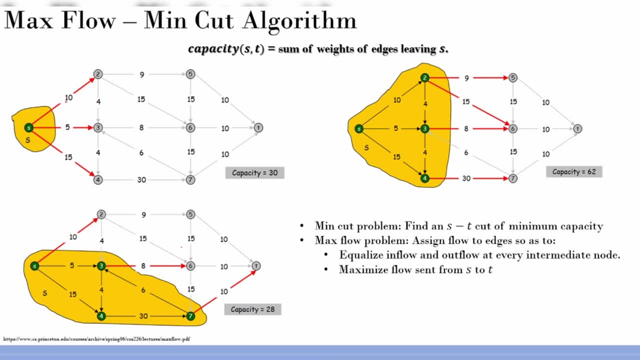 So, whatever that is, that value you choose to go from s to 2 is what known as flow. okay, So you assign some flow, some some flow in that case. okay, So there are several aspects. So you want to maximize the flow. So max flow means. what is the meaning of max flow? 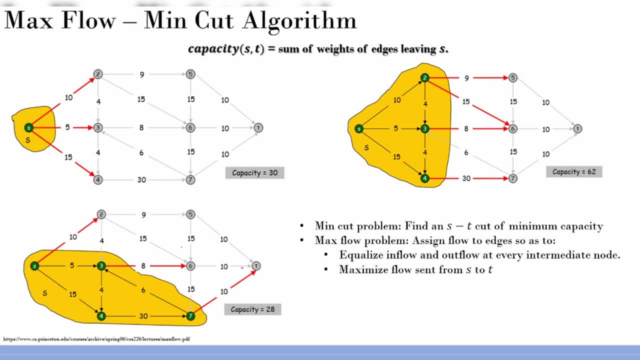 Min cut. I show. I hope everyone understand Minimum capacity cut. okay, So that's it. So in this case this is a minimum capacity cut. Now, max flow means I want to maximize the flow from one source to another target. okay, So in this case I can't go beyond the capacity of the particular node. 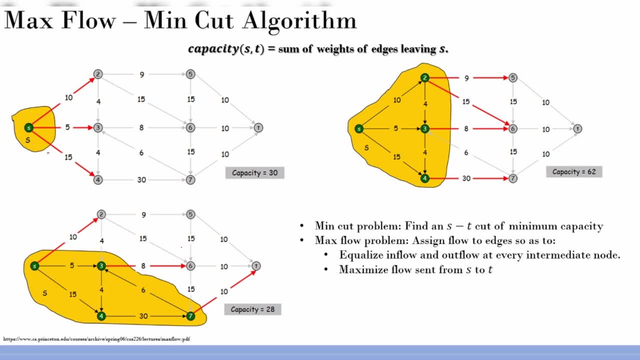 In this case I can't go beyond 10, but I can go between 0 and 10. So I can vary across these three edges and vary the flow such that I can give maximum flow to the other. But there are certain conditions to be satisfied. 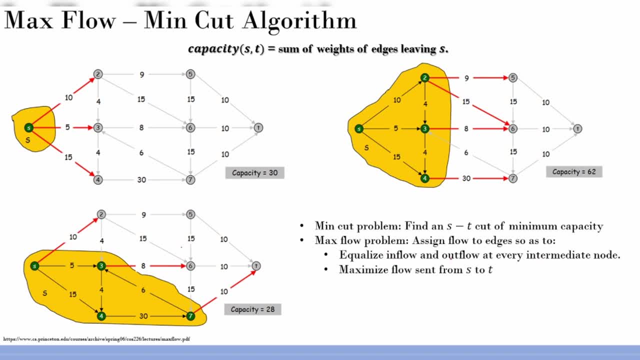 One condition is like inflow and outflow at every intermediate node should be equal. So, for example, 10 is coming here and 9 is basically going here, and there is a capacity to go 4 here, 5 here and 15 here, right? 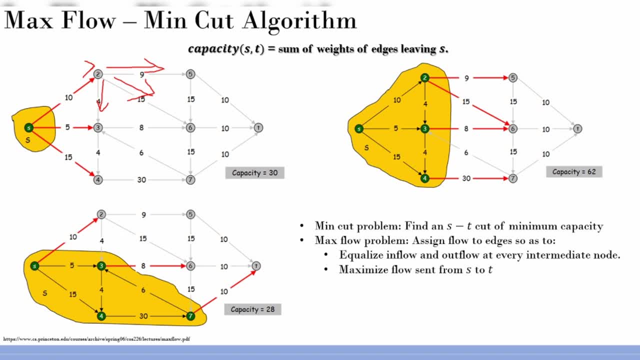 So, but 10 is only coming, So that's a tricky part, So you have to actually balance it out right. So that's the beauty about it. okay, So many places, I think. let me take a better example to show you that. So yeah, I think we can see this way. 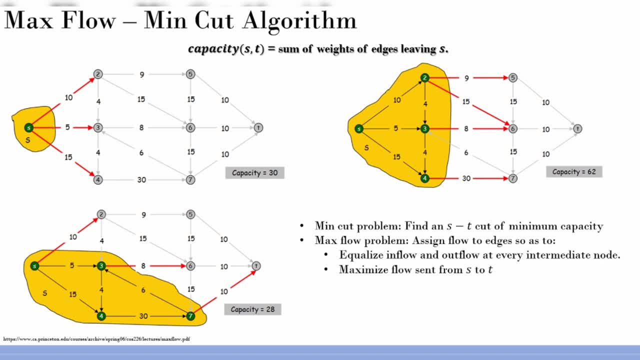 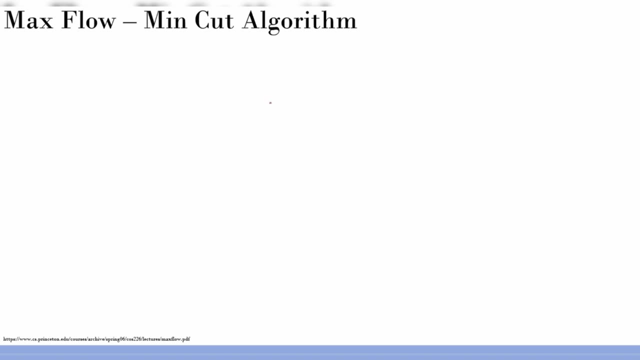 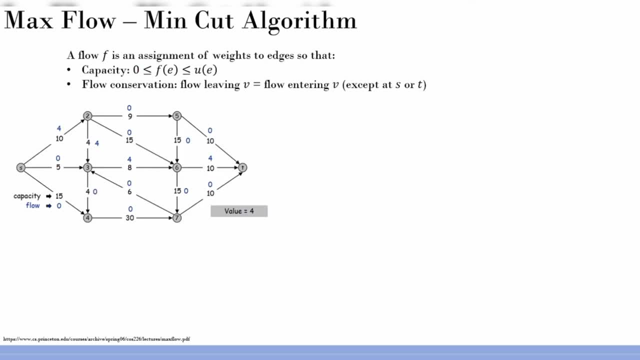 So that's what I have already explained. So we can go the that the capacity is there, so we can actually use that entire capacity for the flow. but we can go anywhere between 0 and the capacity, And then this concept has to be satisfied. 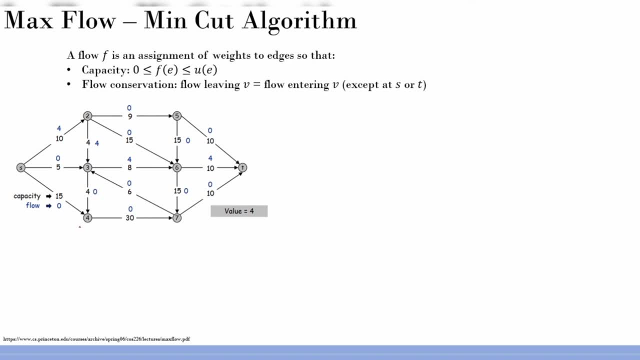 The inflow and the outflow should be same. So let's example. I will explain. So this is the capacity, so 10 is the capacity, 5 is the capacity and 15 is the capacity. Out of that, I am going to only send 4,, 0 and 0 in this case. okay, 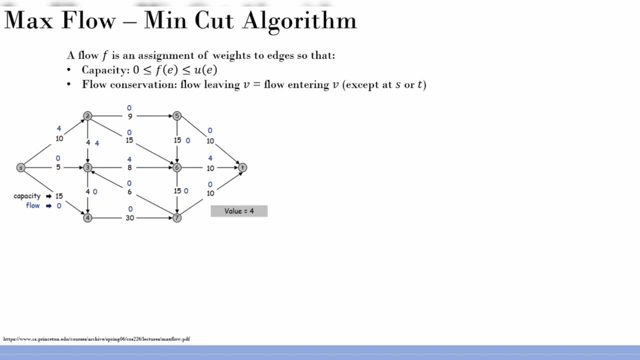 So let's discard it again. So what happens is: 4 is coming here, then only 4 can go out. okay, nothing more than that, Even though the capacity is 4,, 9,, 15, here the 4. if we are planning to go through this. 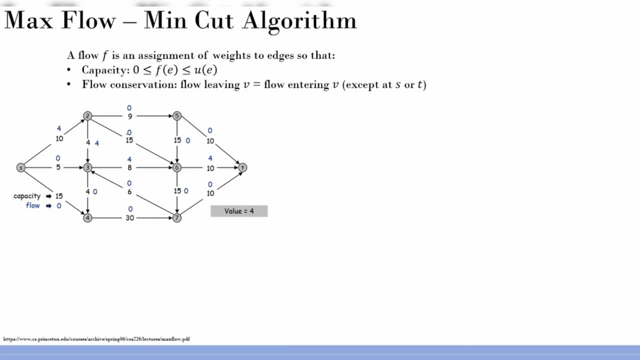 then this has to be 0, we have to balance it out, okay. So that's the thing I was talking about In this case: the flow. the flow in this case is 4, because this 4 plus 0 plus 0.. 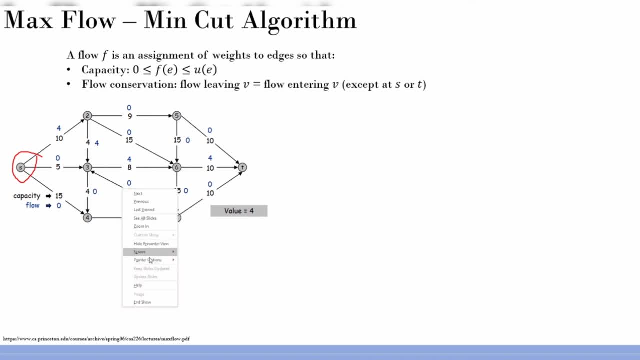 So for this particular guy, this is 4 plus 0 plus 0,. that's it, okay. And now let me take another example. okay, So in this case the value is for this particular source is 10 plus 3 plus 11, which is 24.. 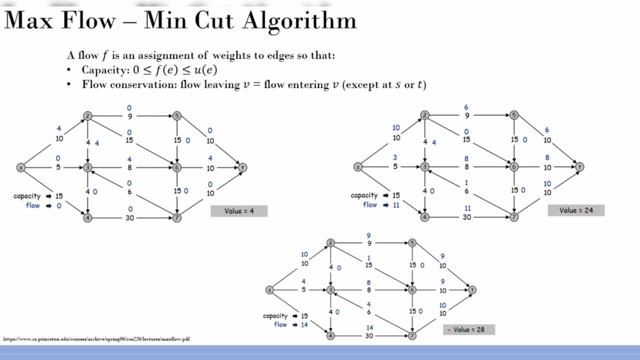 And in this case, for example, is 10 plus 4 plus 14, which is 28,. okay, So three cases I am showing. Now let me go back and combine both capacity, So I hope. So the flow is clear to you. 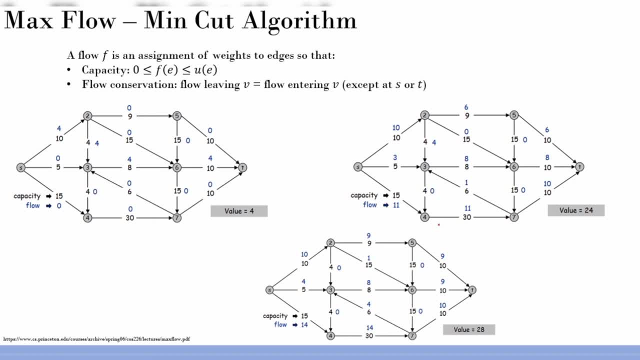 You decide the flow and which one actually has the maximum flow that you should choose. Now it is a trade-off. if you consider both of them together, It's max flow and min. cut both of them together. If you do that, then it's like you have to maximize the flow. 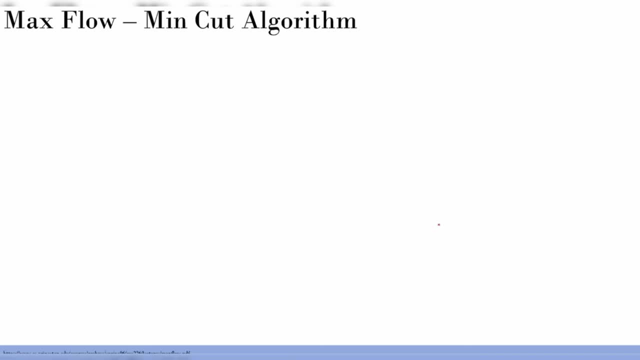 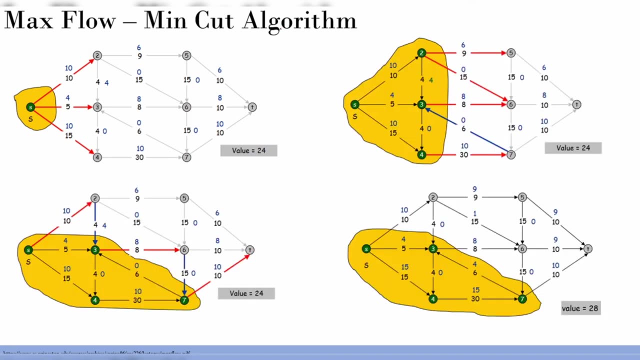 At the same time, we have to minimize the capacity. okay, So that's the thing. Let's assume some examples here. okay, So let me just put all the different graphs here. So obviously, this we already saw in the earlier chart. 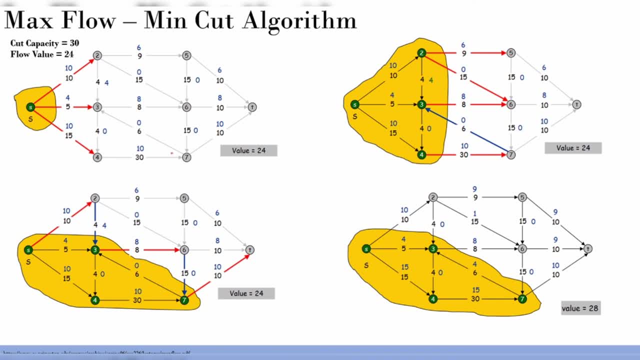 So the capacity Capacity here is 24.. Okay, let me just run it through. okay, So the cut capacity if I actually use, If I want to cut the graph into something like this, so this belongs to, let's say, background. 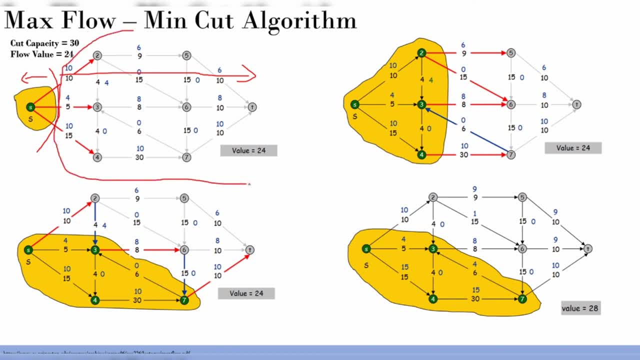 and this belongs, The entire set belongs to the entire Entire, this set belongs to the foreground. Then, if I do that, the cut capacity okay. the cut capacity is given by 10 plus 5 plus 15, which is 30 here. 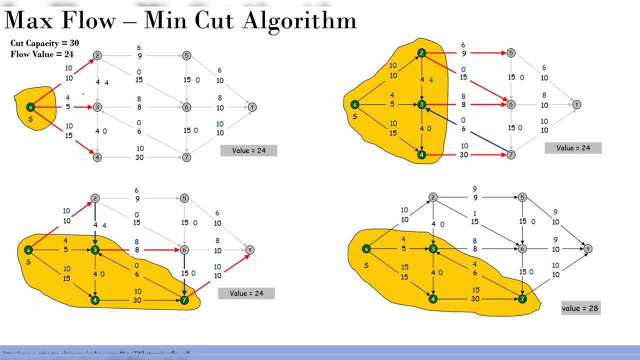 And the flow is 10 plus 4 plus 10, which is 24 here. okay, So that's the case. In this case, for example, if I do a cut like this, this belongs to background and this entire section belongs to foreground. 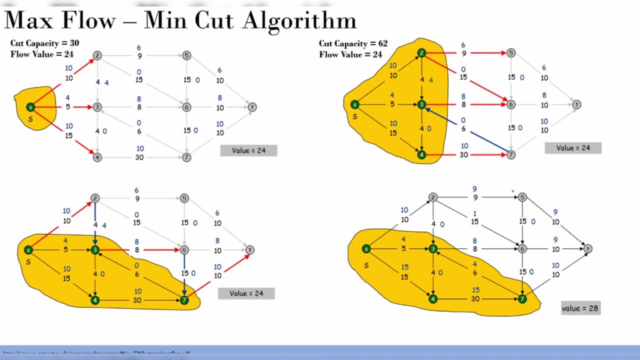 If I do that, the cut- Sorry. The cut capacity is 62,, which again is governed by this particular guy- 9 plus 15 plus 8 plus 6 plus 30,, okay. So 62. Flow capacity is 10 plus 4 plus 10,, which is 24, okay. 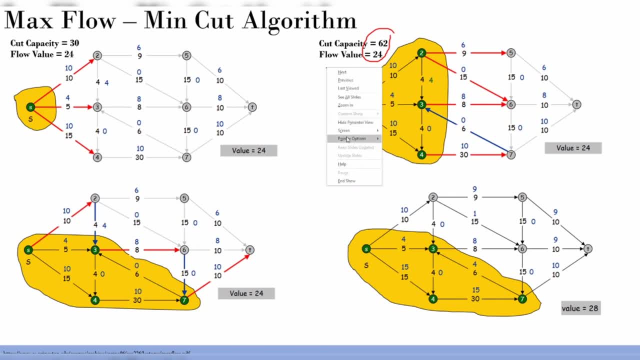 So that's what you're seeing over here. okay, So these two values, And here, for example, if I go, This will be 28, which is again given by 10 plus 8 plus 15, okay, Is not it correct? 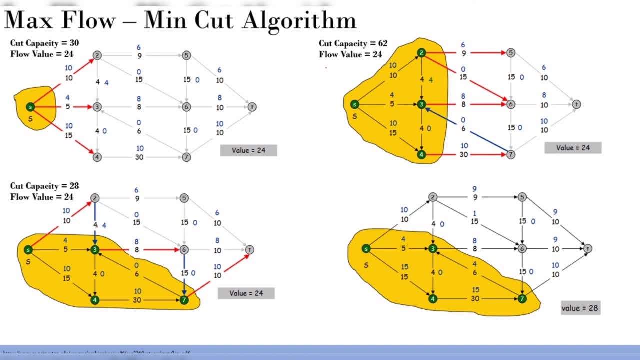 Yeah, Sorry, Yeah, Yeah, So sorry. This 10 plus 8 plus 10, right, that is 28 is Sorry. Let me just Sorry, Okay. So what I'm talking about- cut capacity- is this 10 guy? 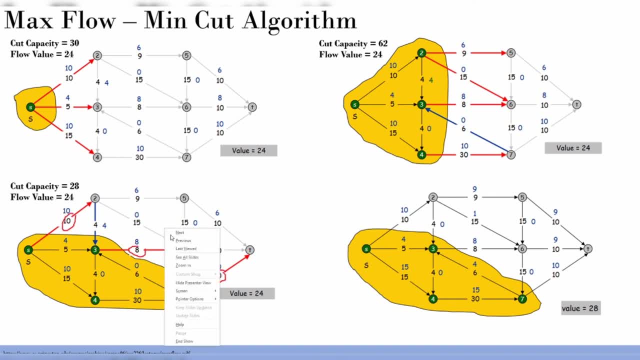 plus this 8 guy, plus this 10 guy is 28, and the flow, if you calculate otherwise, will be 24,. okay, So 10 plus You consider all the flow, then it will come to. You have to subtract, right. 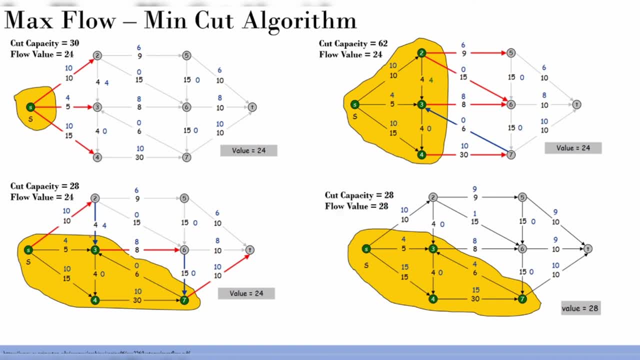 If flow is inside it will be minus. okay, So you do that, you get 24.. And then here if you see it will be cut, capacity is 28, and flow value will be 28. And obviously now you can. 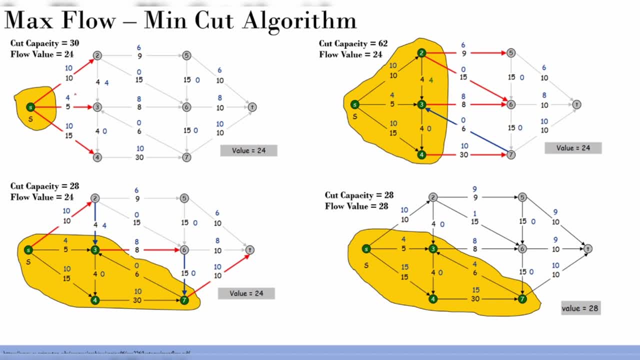 So what we did, just to reiterate, don't lose the higher picture. So you converted your image into graphs, into knots and edges, And once you do that, you treat it as a graph cut problem or a max flow mean cut problem, like this: 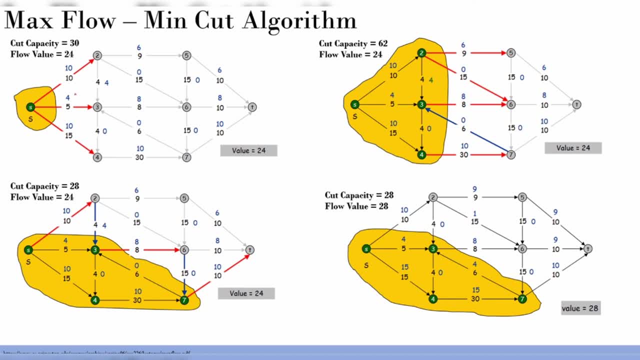 So, for each particular thing, the algorithm. So it's a very complex algorithm. You can think about it. It will calculate the cut capacity for various possibilities as well as the flow value for various possibilities, And then, of course, you do consider both the values together. 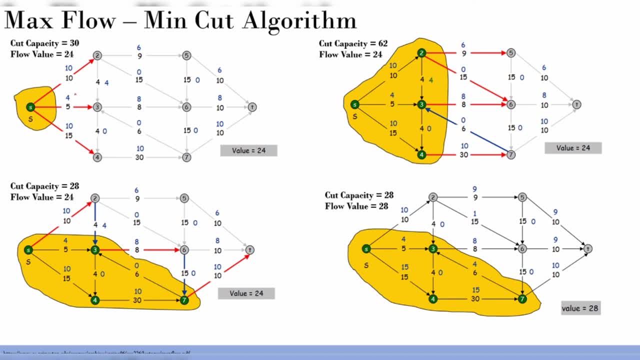 and you want to maximize the flow. At the same time you have to minimize the cut capacity. So in this case, obviously all the values are in front of you. You are bound to choose this guy right, because it maximizes the flow- value 28.. 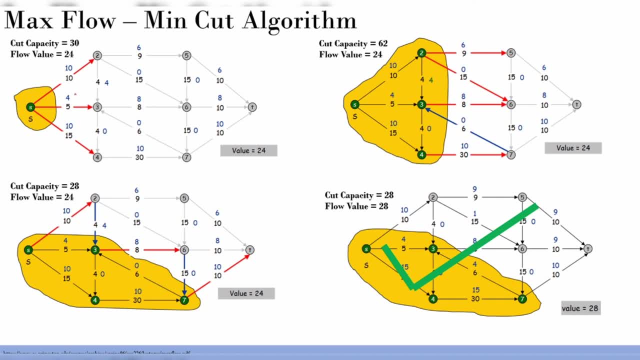 That's a maximum possible. At the same time, the capacity is sort of a good trade-off, right. You can even choose this one. It's not a bad result here, but you will go for this, And if you do that automatically, you are bound to get the best result okay. 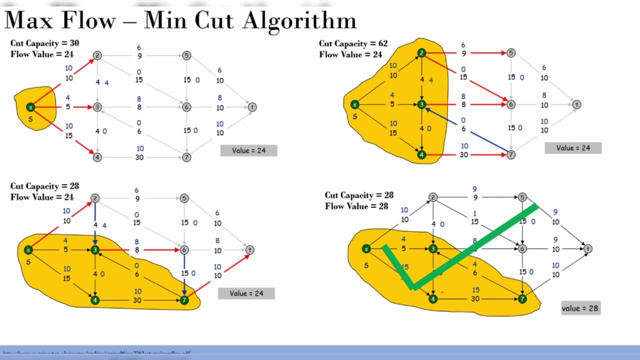 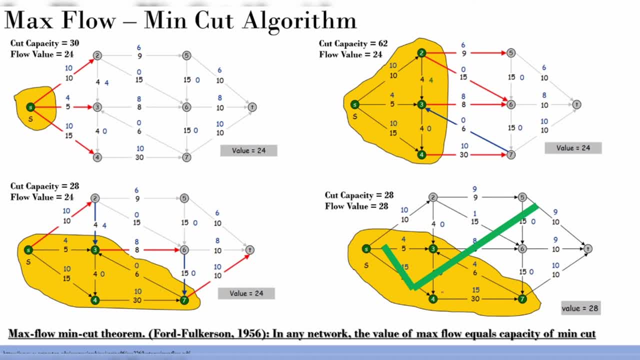 if you study graph theory, if you study graph theory, if you read it, you might have heard about it. It's a Ford-Fulkerson algorithm. So if you are more interested, please, of course, go through that classical paper in PAMI. 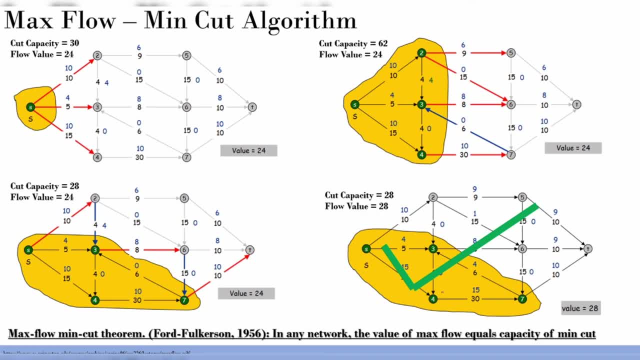 You'll get more details about it. okay, So this is how you approach the problem in graph cut, And with that we are almost over with the lecture in this week. okay, So we discussed in last the graph cut algorithm, which is sort of taking from the graph theory all the concepts. 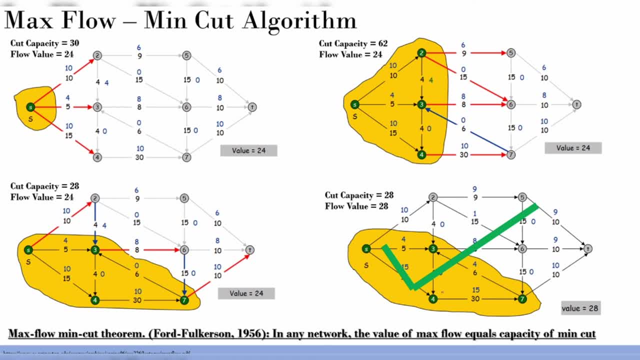 and using it in image processing, right. So that's the beauty about this technique, okay. So that's the beauty about this technique, okay. So I hope I'm not confusing you, but all these are available as a sort of an API to you. 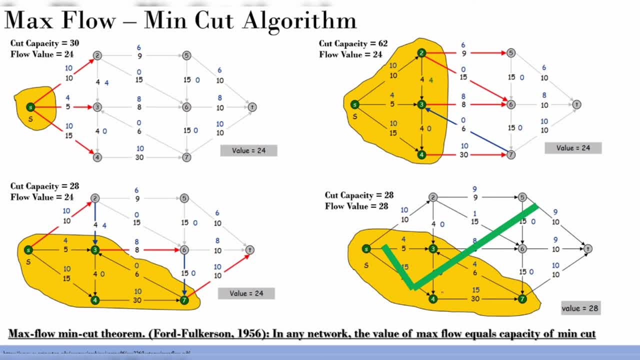 So you don't need to really develop all the algorithm, but I will give a MATLAB code, which will take a lot of time to run because it has to go through all these right. So it takes a lot of time, but you can have a feel of what is happening inside, okay. 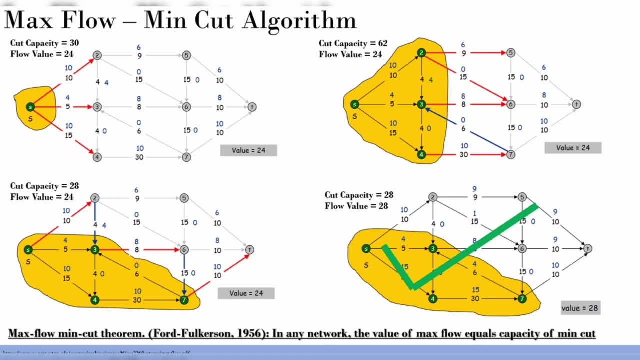 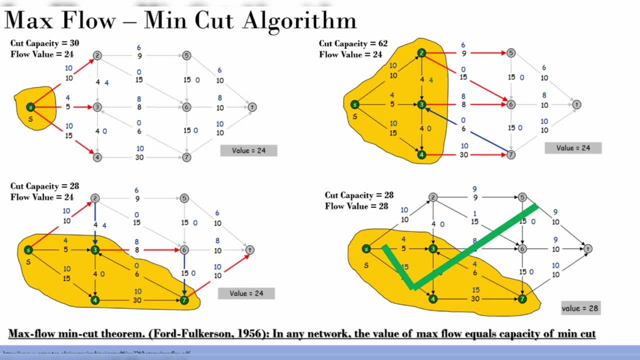